I am very happy to be able to share this webinar with you. It is a pleasure to have you here. Thank you, And we appreciate your attendance. We are happy to have you here, Thank you, Thank you, Thank you everyone. 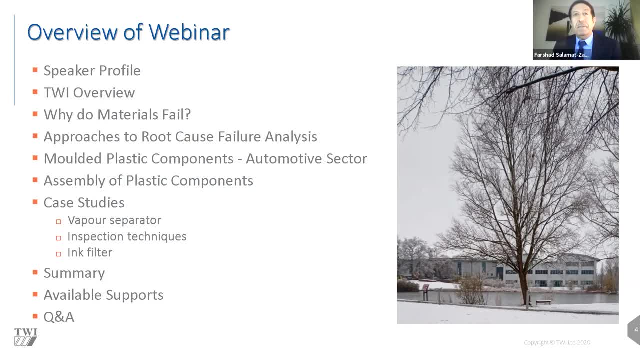 Thank you, Thank you very much, Thank you very much, Thank you very much. challenging time for everyone and I hope everyone is safe and keeping well. The overview of the webinar today is that I will give a short profile about myself and a couple of slides about TWI and who TWI is and what we do. 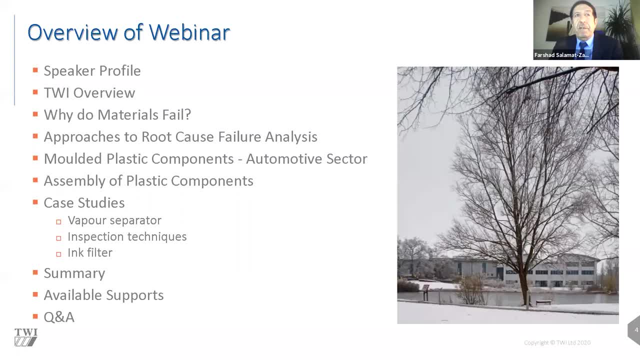 And then I will put the focus on why material fails, different approaches to root cause failure investigation and give examples from the automotive sector mainly, and also the method for joining and assembling of the plastic components. I will present a case study which will go through various laws and various inspection. 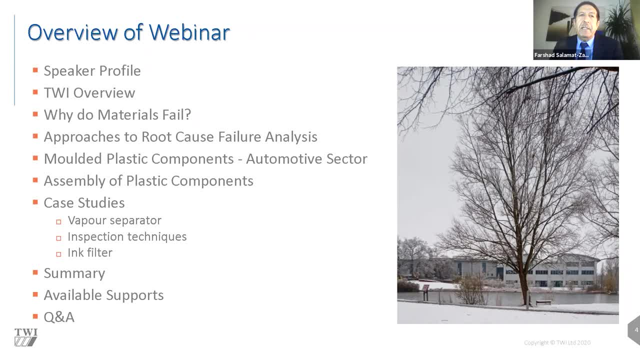 techniques and I will summarize that at the end and provide you with any additional support that we can offer. And there is a question and answer at the end where, as my colleague said, at the bottom of the Zoom meeting, you will have, instead of the normal chat, you will have a Q&A. 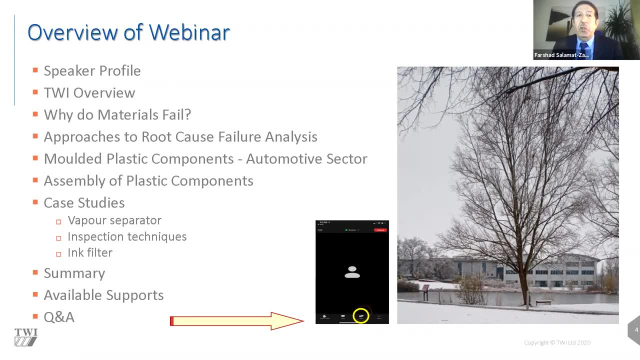 You can write your questions in the Q&A template there and then we will answer them within the timeframe of the webinar at the end. If you don't get the chance to answer all the questions during the time, we will respond to you by email and we will answer your questions there. 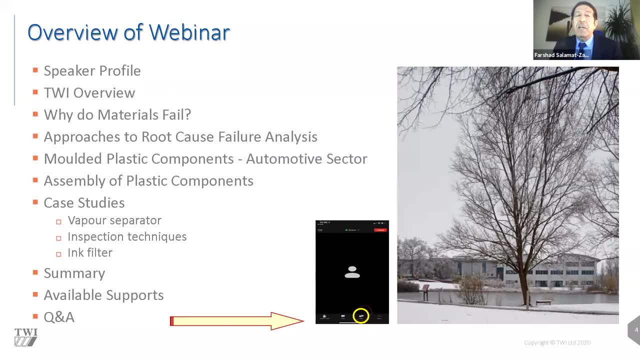 And, as my colleague said, a copy of the presentation will be available to you later on. My colleague Carol will address that. Thank you, Welcome everyone. I'm going to tell you a little bit about the presentation. I'll start with my colleague Eestion. 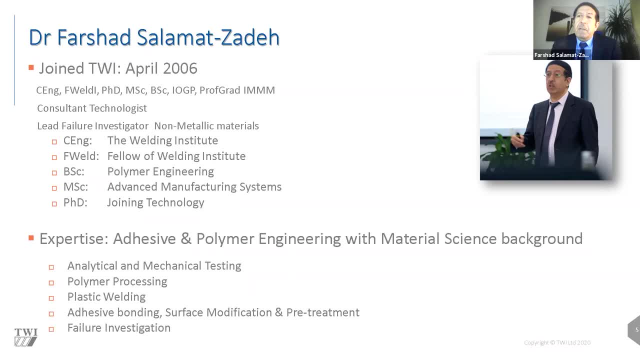 Thank you, Prof El-Massoud. I'm going to start with the presentation. I will ask the question and the answer will be available. You can contact me at the bottom of the Zoom chat And that's the Q&A. 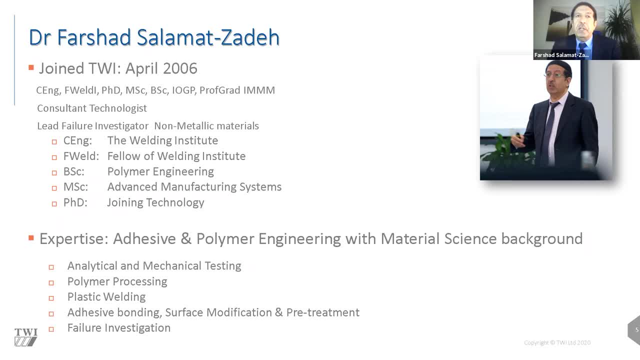 Thank you, Hello everyone, Thank you everyone. Thank you so much for joining our panel technology. My expertise obviously is in adhesive polymer engineering and I've got a material science background as well, But some of my skills include electrical and mechanical testing. 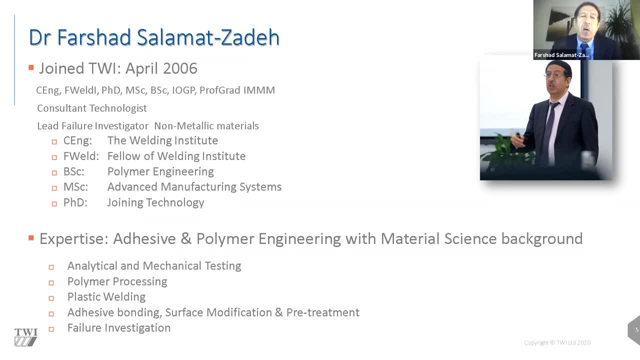 of products and of coupons and all component products, Polymer processing, all the welding associated with plastic weldings, adhesive bonding, surface treatment and pretreatment and so forth. And also 70% or 80% of my time is dedicated to failure investigation. 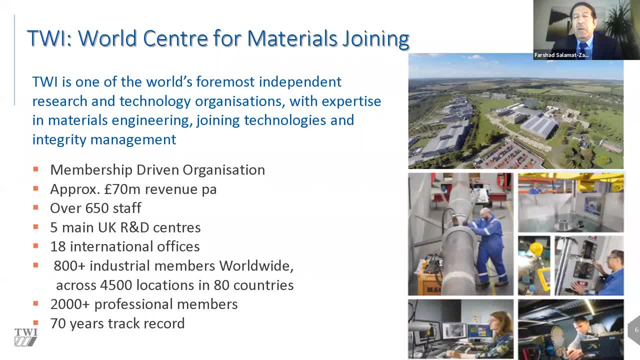 In terms of TWI. TWI is one of the foremost independent research and technology companies globally and we provide engineering, material engineering and welding technology expertise and as well as the integrity management. We are a membership-based organization and basically by that what I mean is that companies become a member of TWI and our services. 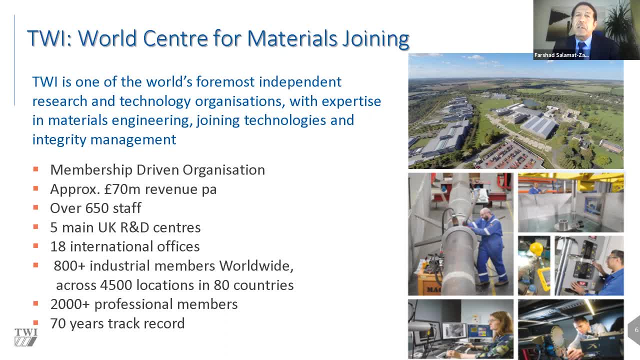 and expertise are dedicated to our members, so we become the extension of their resources, And that's usually. the membership is annually based. We have more than we have- over 70 million pounds of revenue annually. obviously that fluctuates and like everyone else, And 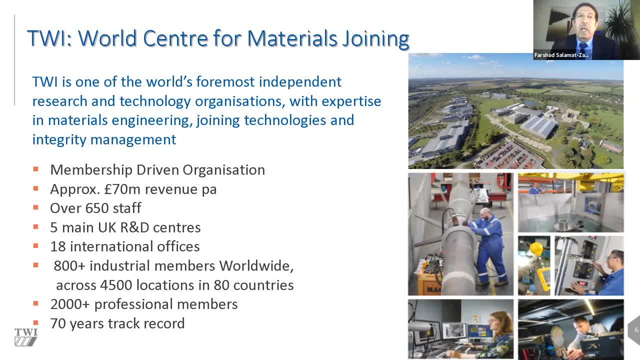 we have more than 650 staff globally. We have five-star staff and the six-star staff are from France, And that's really one of the reasons why we are incredibly popular. We have a lot of people in crane. we have thousands of people in the sector that are working with the industry. 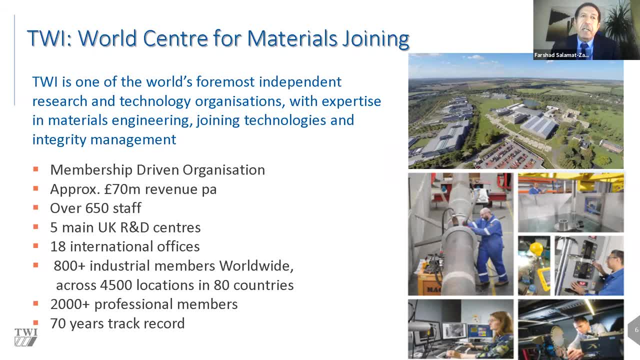 and we have thousands of companies in the industry that are already active, And that's also the sites in UK- five R&D sites in UK, in United Kingdom, and we have more than 18 international offices globally. As I said, we are a membership-based organization. we have over 800 industry members, but they 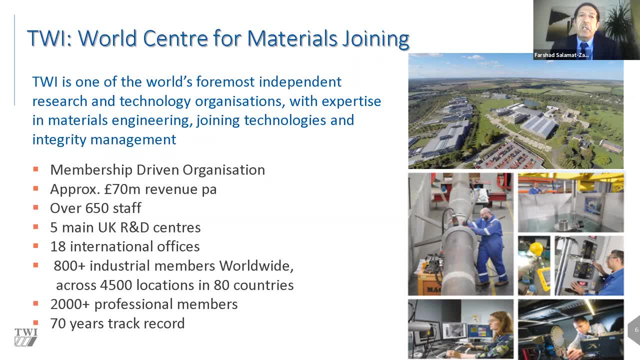 are spread over roughly about 4,500 locations in over 80 countries, so you can imagine the extent of our deliverables to our members. And on top of that we also have over 2,000 professional members, such as the members. 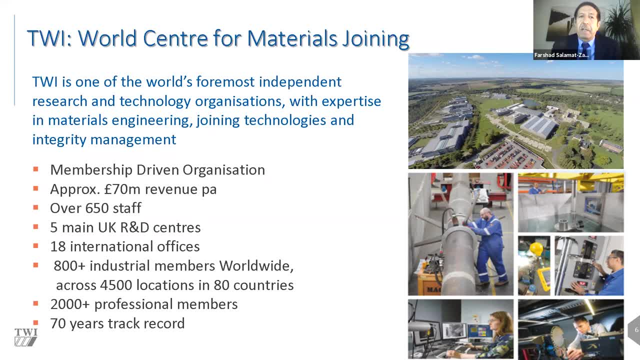 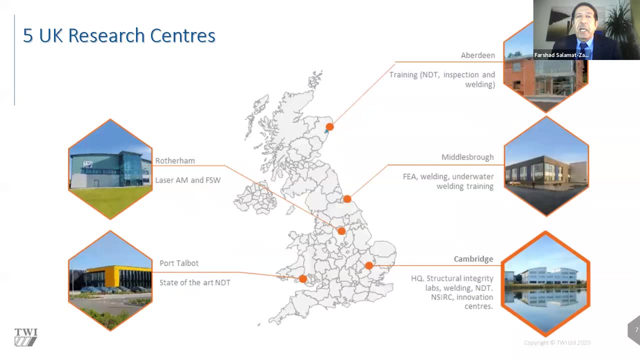 of Welding Institute, the senior members and the fellows and so forth. TWI has got over 70 years of track record and it was set up after the World War II at Cambridge University. I mentioned UK sites, so other sites. 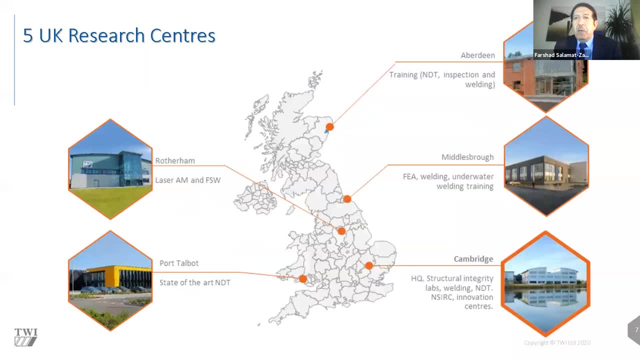 Our headquarters are in London and we have over 1,000 international offices globally. Our headquarter is in Cambridge and where most of the laboratories are there, the Asset Integrity is there and also quite a big chunk of our non-destructive examination center. 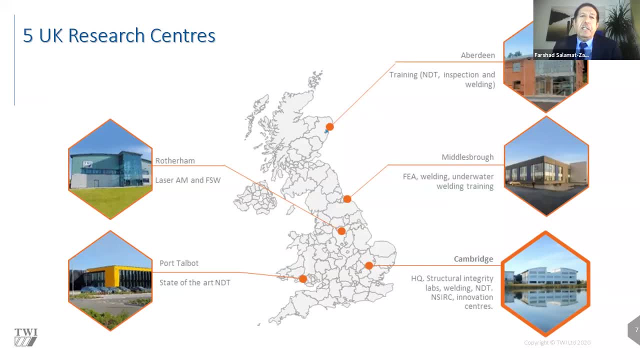 And we also have NSERC, which is National Structural Integrity Research Center, as well as the Innovation Center and as well as the Non-Metallic Innovation Center, which is another division of the part of the Innovation Centers. it is there as well. 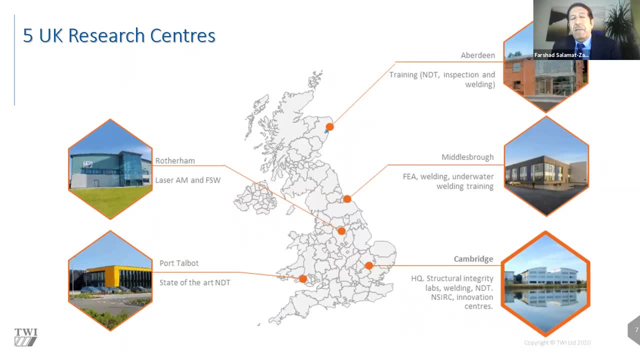 In our Middlesbrough sites we have modeling, final element modeling. we have welding and underwater training, welding training courses and in our Aberdeen is more of an office space but again a lot of the training is carried out there for the, which is dedicated to oil. 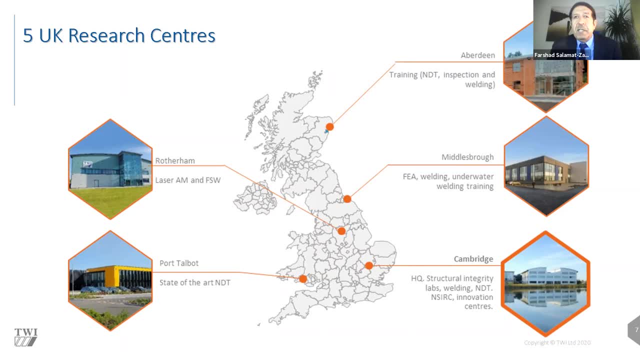 and gas sector. In our Rotterdam, which is near Sheffield, we have our laser additive manufacturing and friction welding technologies based there, and in our Port Talbot in Wells, we have a state-of-the-art NDT again which is as I said, it supplements what we do at TWI in. 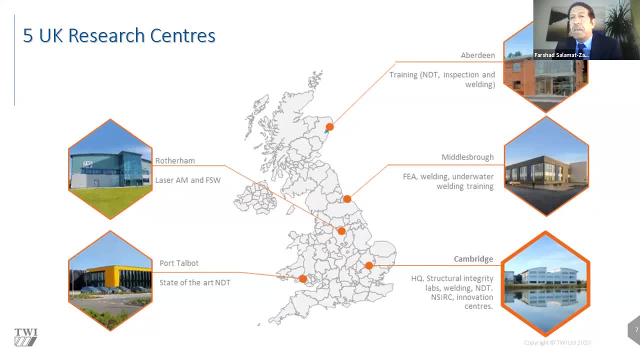 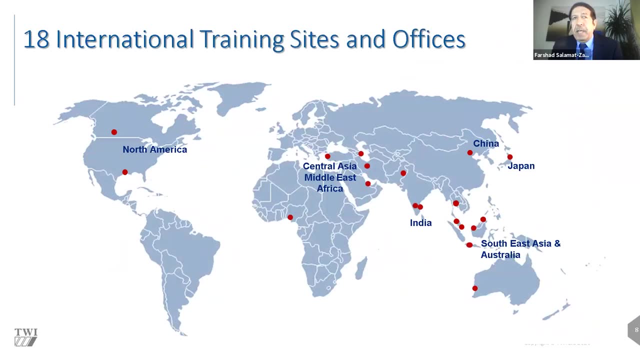 headquarter and also they work as a big team there. Globally, I mentioned, we have more than 18 offices and training centers from Canada and US to Europe and to Middle East and quite a lot in, obviously, in India, China, Malaysia. 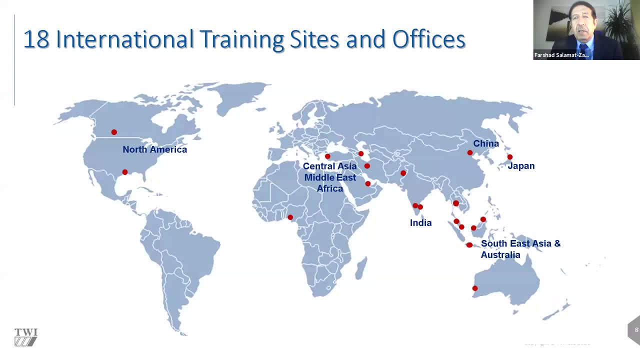 and so forth. So we have good presence, good footprint. Thank you. We also have some really good connections across a number of key areas. In the countries where we don't have offices, we have agents who act on our behalf and they put clients in contact with us and we address their needs that way. 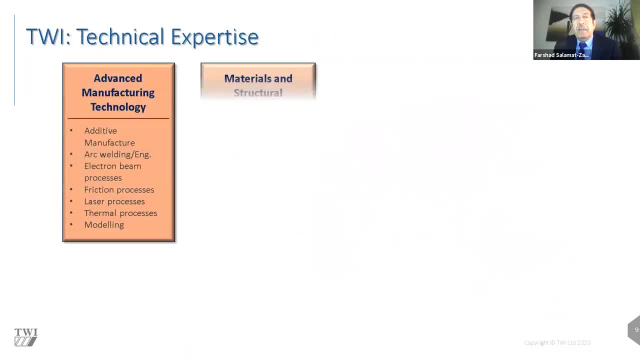 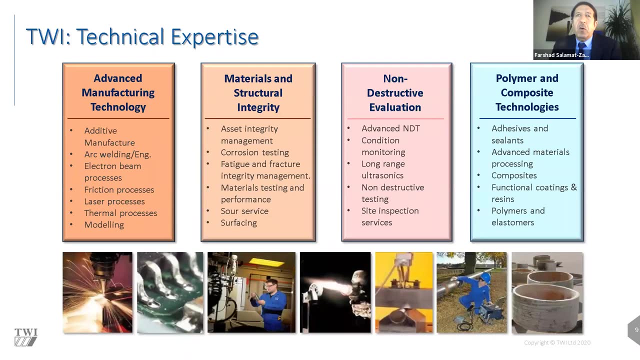 In terms of the expertise that we provide internally, we have divided our capabilities or expertise into four groups: Advanced Manufacturing Technology Group, material and structural integrity and non-destructive, and also the polymer and composite technology. so there are four groups and i myself. i sit in the in the polymer composite technology. 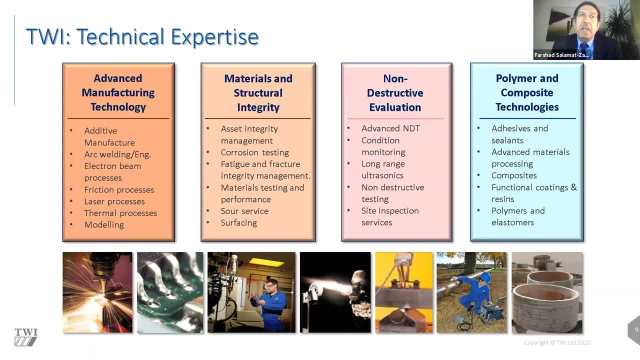 group and you can see from from the list, each group has got certain certain departments or sections within them which is a advanced manufacturer. you can see that we are involved with additive manufacturing, arc welding and associate technologies, electron beam welding processes, friction welding processes, laser and laser welding, thermal processes and final. 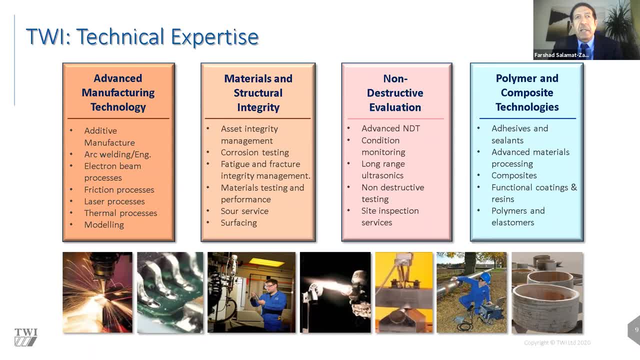 element modeling as well in the material science, in the material and structural integrity, asset integrity management, corrosion, fatigue and material testing and performance. and also the sour services for the oil and gas sector, also the surface engineering, are residing under that group And non-destructive- we got advanced NDT section. 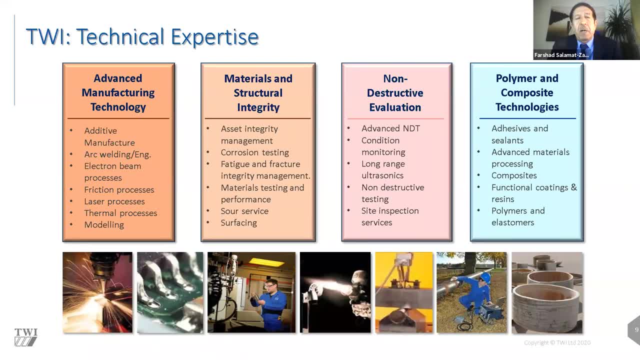 sitting there and we've got the condition monitoring. long-term long range ultrasonic testing and site inspection and so forth are sit under that flagship And in the polymer and composite technology group we have we provide adhesive and sealant technology and expertise there, advanced material processing. 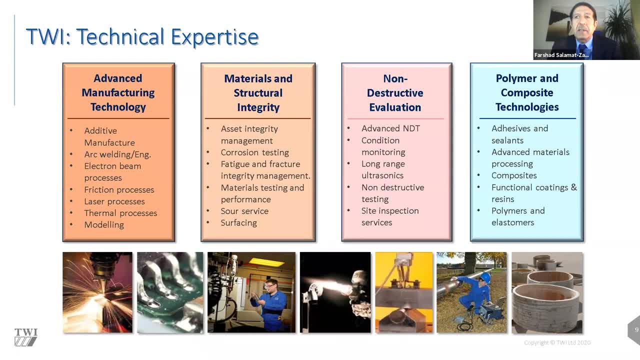 composites and functional coatings and resin system, and also the polymer and elastomers are on. they sit under that group. So we provide, you can see from, we provide whole range of technologies in terms of processing, in terms of joining technology and also in terms of material engineering. 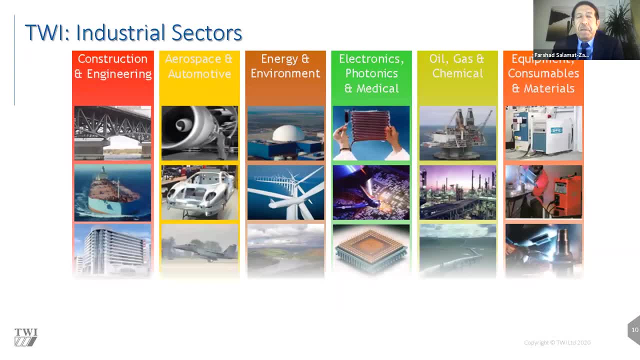 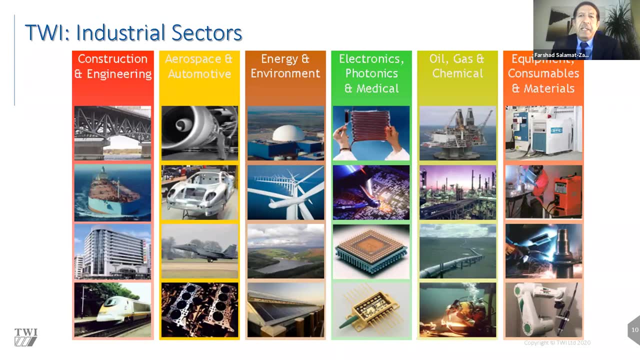 across the various groups In terms of the industry we serve. basically we serve all major industry sectors and internally again we divided them to six groups, which is construction and engineering, aerospace and automotive, energy, environment, electronic, photonic and medical sectors. 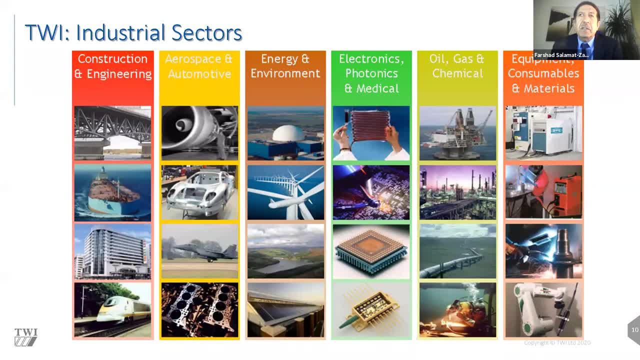 and also oil and gas and other affiliated chemical industries and equipment, consumables and materials. So under each of them obviously they cover whole range of industries and companies that that system. So we, we divided. as I said, we divided up to six groups. 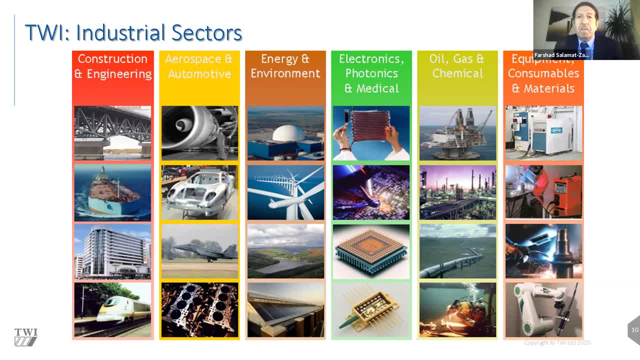 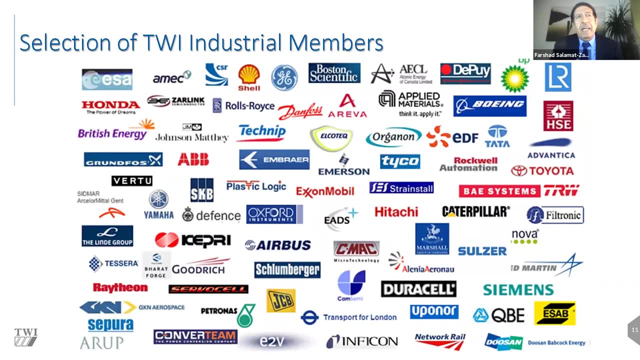 and we provide the services to all, to all those sectors. That's the kind of a general background about TWI, and a selection of other members are displayed here. As I said, we have over 800 plus members and it's not feasible to put all of them on one slide. 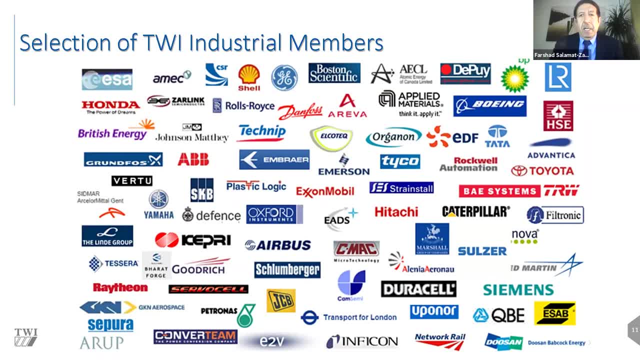 And at the same time, I have to emphasize that some members they prefer to be a stealth member. So basically they use, they are our member and we provide services to them, but they do not want us to disclose that they are members. 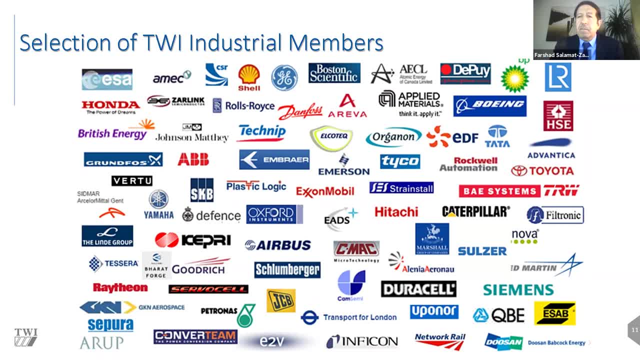 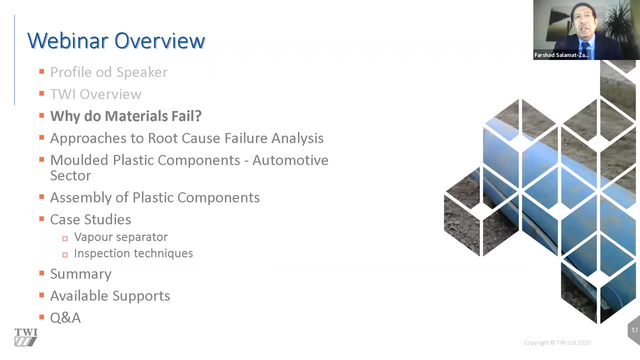 So there are certain members fall in that category, but a selection of the members are listed here, So you can see the diverse range of membership portfolio that we have Now going to. the topic of the discussion of webinar is the failure investigation And the welding of the molded plastic component. 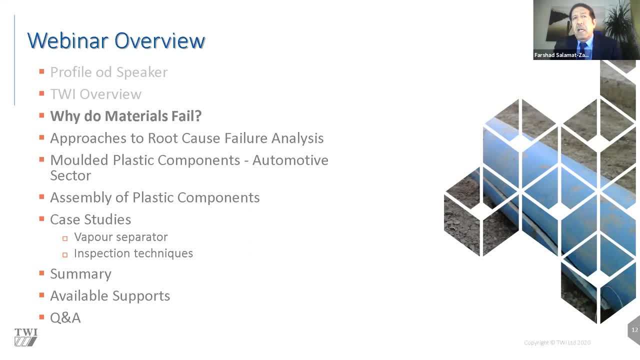 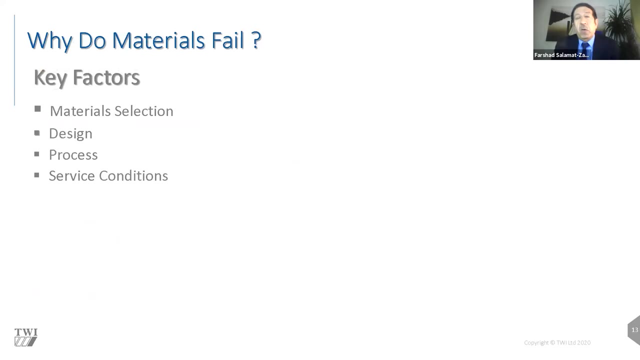 So initially the first question is that: why do materials fail? And then, once we start looking at that, then we can start answering other questions that follow. But why do material fail? The key factors really is can be summarized in four sections, in four categories: material selection. 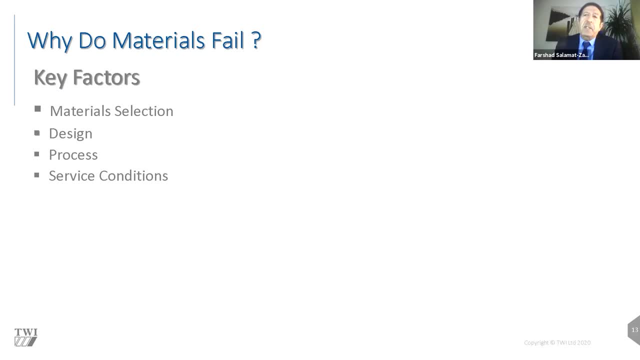 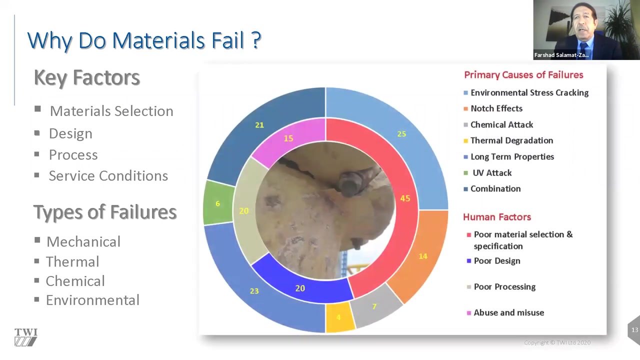 it could be design factor, it could be the processing factor or the service conditions. And the type of failures. it could be mechanical, due to mechanical failure or thermal aging, thermal degradation, chemical attacks, environmental attacks, But these are some of the causes of them. 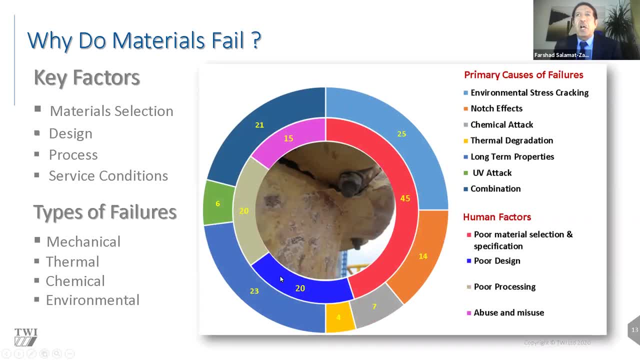 And now what I've done here. I'm trying to portray the primary cause of failures, and also so the outer ring refers to primary causes of failure and the inner ring is the percentages related to human factors that lead to failures. So, in terms of the primary cause- failures- 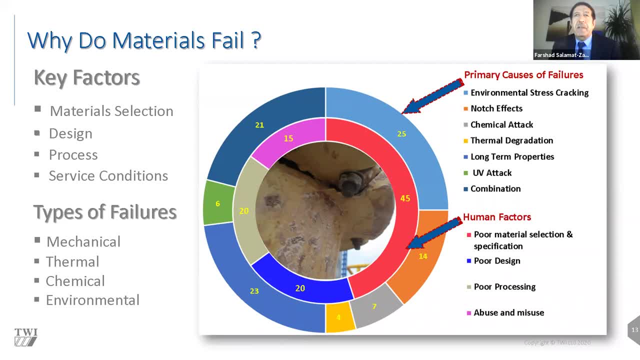 you can see from the outer ring, environmental stress cracking, for example, that that's about 25% of the overall failures. and notch effect: chemical attack, thermal degradation, long-term properties, UV attack and combination of some of one or two or more of these. 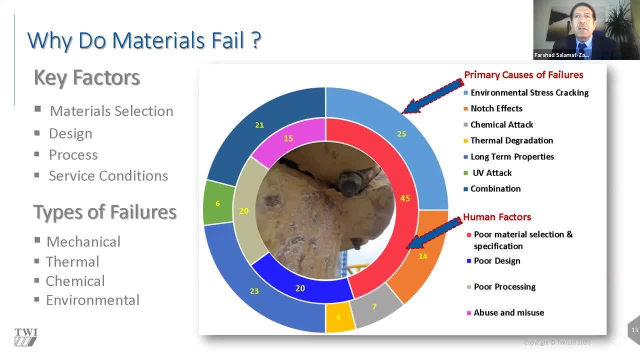 these causes are also about the same, So it's about 21% of the total failures In terms of the human factors, for material selection or specification by designer, for design, for design, and then whether it's for the welding, for the joint design itself. 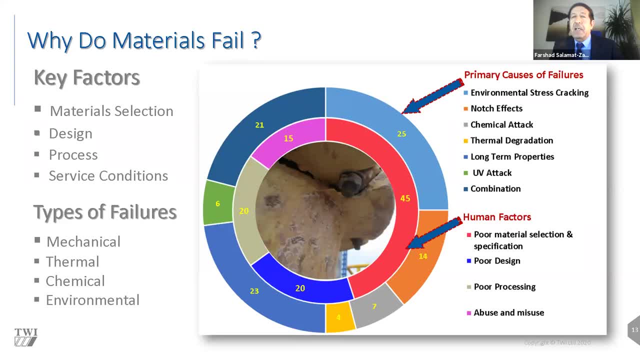 or whether in terms of the material and the component to be fit for the purpose, and also the abuse and misuse by the people who's handling it, For example, if you're talking, for example, about a sort of headphone or an office chair. 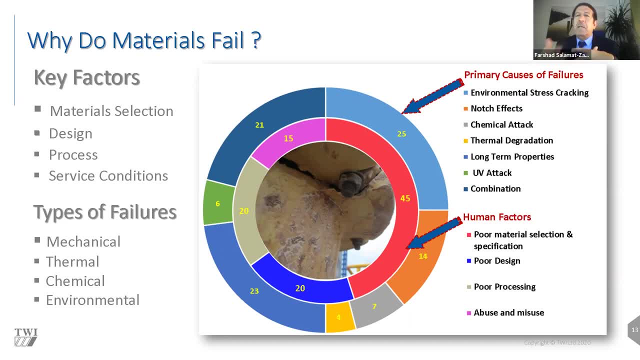 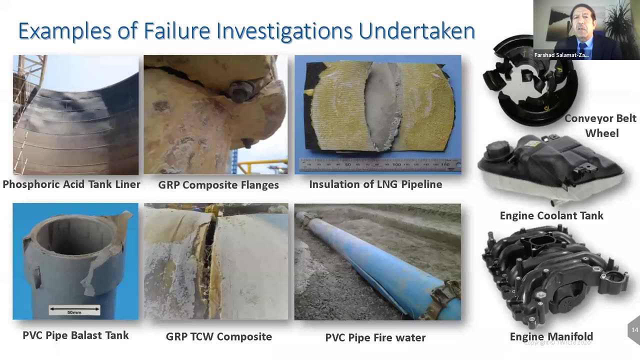 it's a way that person interacts with that device can be a misuse or abuse of that product, So they fall under that category. In terms of some of the examples of the type of work I've been involved with, I've been involved with more than 320 different. 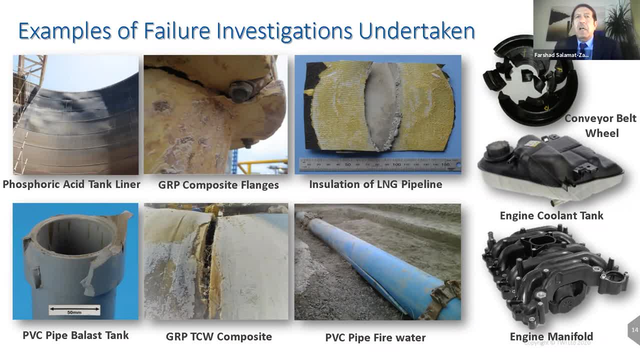 data investigations. Just a sample of them are highlighted here: For example, the liner, the phosphoric acid tank, for example. that was a site inspection and it involved a lot of on-site analysis and then back to the laboratories: GRP composite flanges. 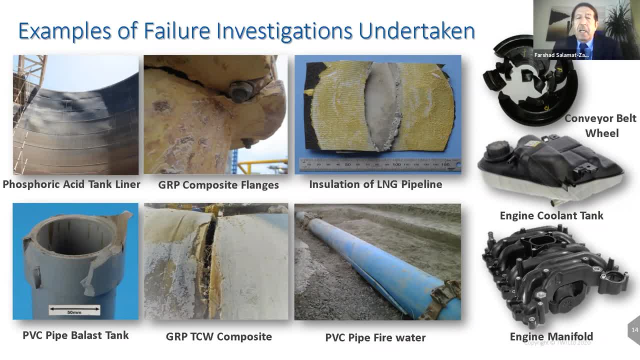 and all the insulation of the LNG pipelines and the fracture of the failure or explosive failure of the PVC pipes in a tank blast ballast tank of a ship and the failure of the composite pipes in the oil and gas sector, for example. 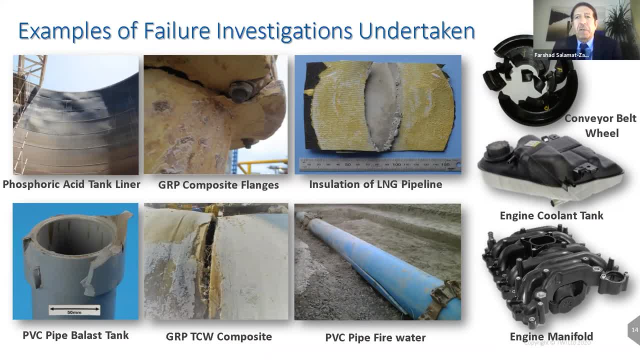 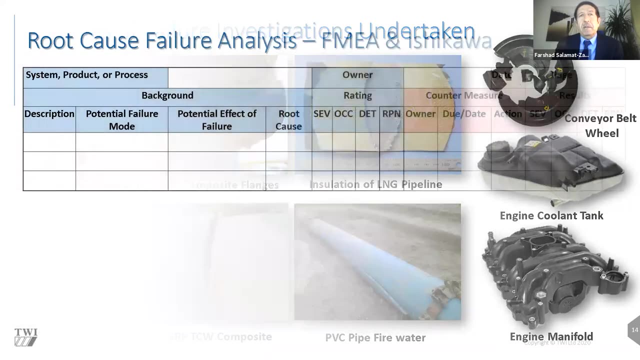 or water utilities, PVC pipe for fire, water again in refineries, and a lot of the molded components, both for the automotive, consumer good materials and so forth. So how do we go about carrying out failure investigation? There are a number of techniques. 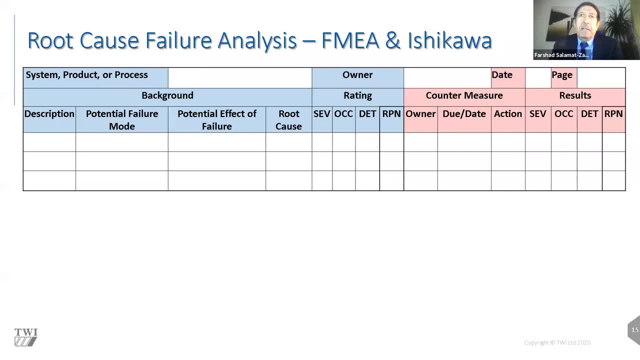 and one technique is obviously is a failure mode and effect analysis, Which this kind of diagram, this table, is an example of such a process. Different companies, they develop this table differently for their own use. Basically, we have to identify whether the failure 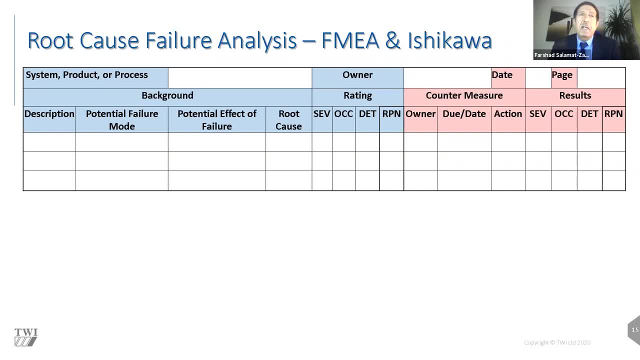 is a system failure, whether it's a product failure or whether it's process failure, And then from that we got to provide a description of it, potential failure modes, the potential effect of that failure, that we can have The root, try to identify the root cause of it. 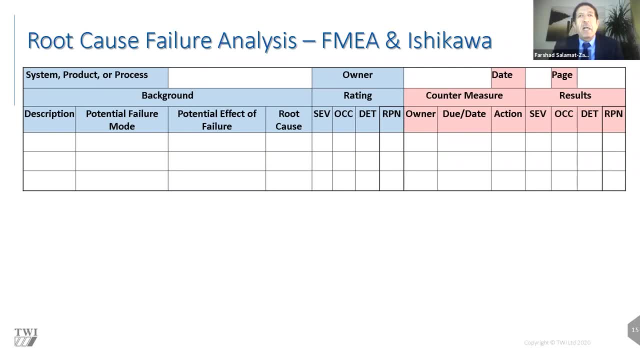 And then, in terms of the rating of it, giving a number to it, then we need to know the severity of it, the occurrence of it, the detectability of it and obviously the risk, And then we associate the risk number with that type of failure. 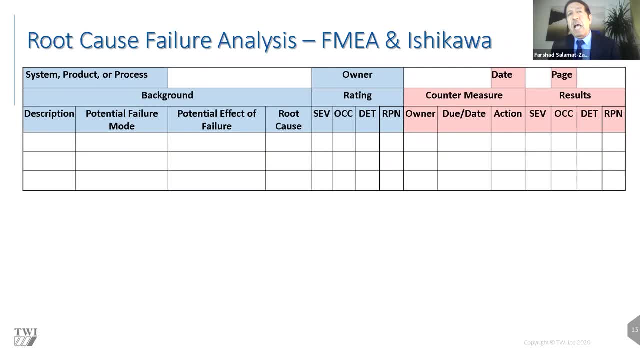 And then for any failures, obviously in terms of the countermeasure, how are we going to resolve that failure, identify the root cause and put the right measures in place in terms of, obviously, somebody needs to take the ownership of it, And then there will be certain actions. 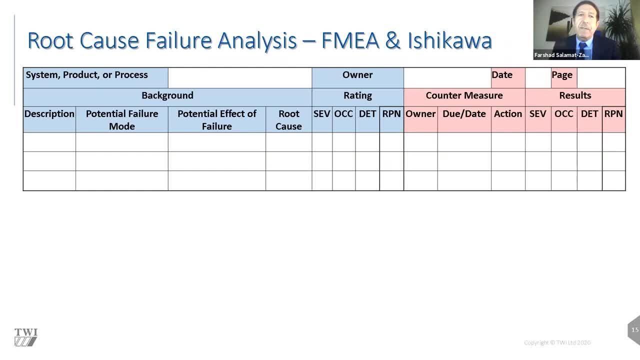 And then, based on the actions, then we look at again, we look at the severity, the occurrence, detectability and also the risk associated with the risk number, so that we can try to see whether we have implemented the right countermeasure for that. 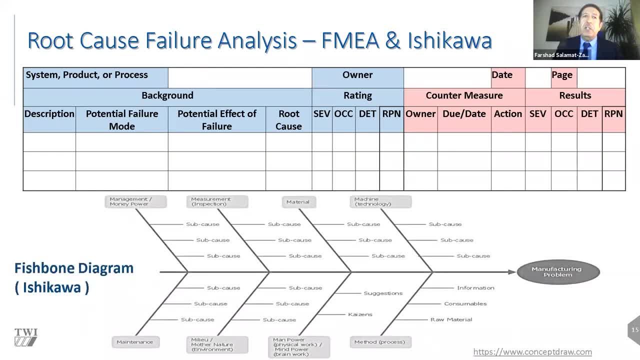 Another technique is also used in industry is the Fishbone Diagram or Ishikawa. Again, this is just an example And basically, taking example of manufacturing problems or taking example of manufacturing problems, we can associate different activities. It can be associated with the machine. 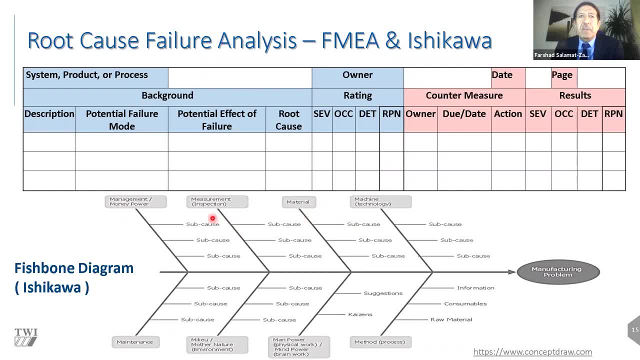 or it could be the materials, It could be the type of inspection and measurement techniques, or it could be to the manpower, It could be maintenance associated failure. Maybe the maintenance wasn't carried out regularly, or maybe it was missed, or things like that. 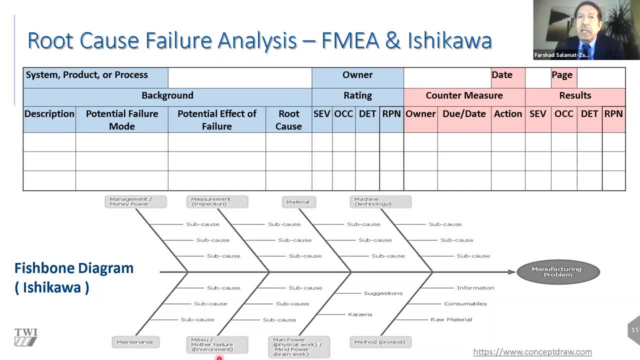 Or it could be environment, modern nature and so forth, Or in some cases it could be obviously the mind power or the manpower, and then obviously we use techniques such as Kaizen to assess that And again in terms of the methods or processes, 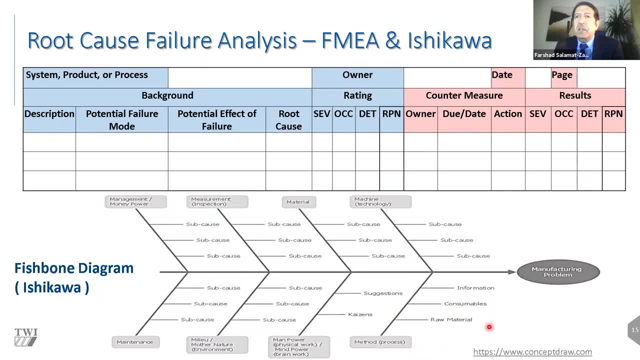 it can be areas such as raw material and consumables and so forth, But there are obviously areas, all of these side branches or sub-causes for each product, for each process is going to be different, So we need to identify. 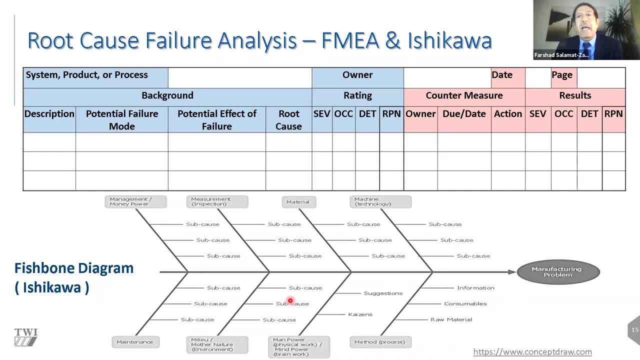 So a team of engineers, when they're doing the root cause failure analysis, they go and start populating this and be trying to, with that, identify what hasn't been done rightly and then try to identify and then put the right countermeasure in place to resolve it. 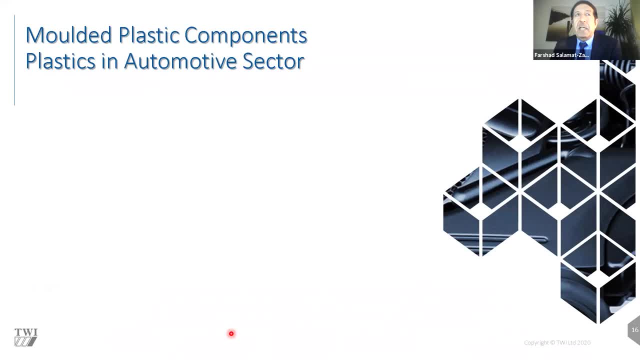 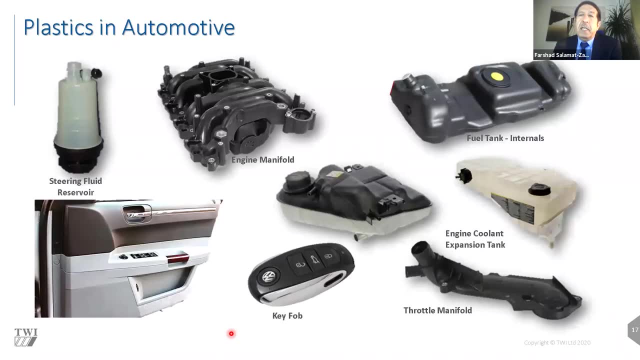 So the topic of the webinar is molded plastic components, And I give examples of various automotive components that I've been involved with, and they vary from a lot of different pressure vessels or maybe even engine manifold And fuel tanks as well. again, it gets pressurized. 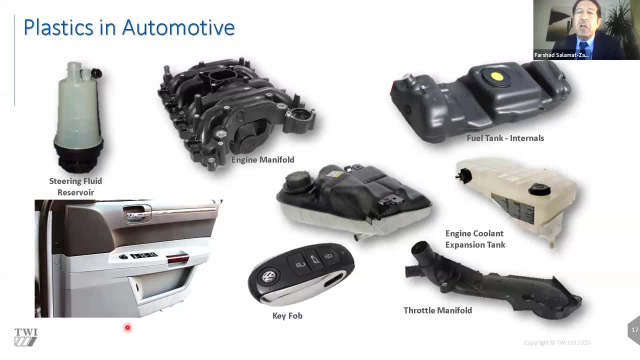 sub-components fit in the door or in cabin of the car. Basically, as you can see from most of these examples, these are. they are made from at least two different halves, So they are molded. they are complex shaped. they are molded injection molded in two halves. 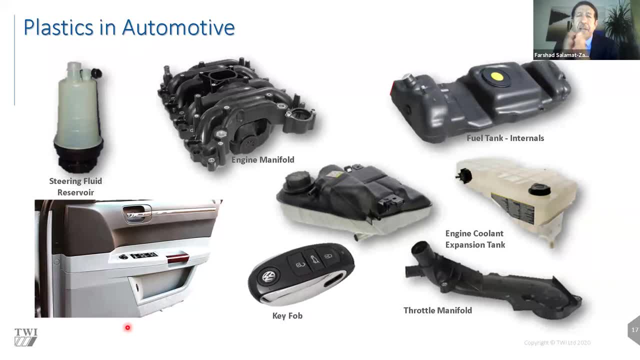 and then they brought together and they got to be assembled. So where they are assembled or where they are joined by welding or by adhesive bonding, that's sometimes that's where we get the failures, and then we need to investigate why those failures. so these are just some examples. 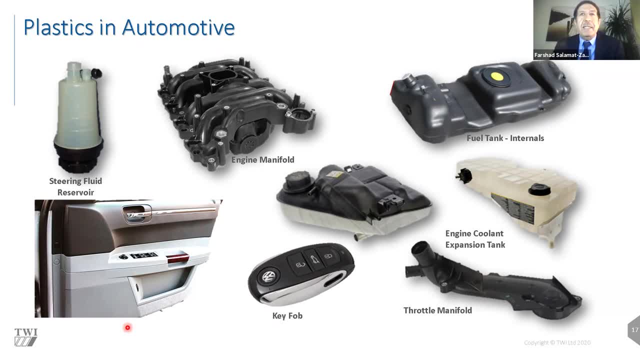 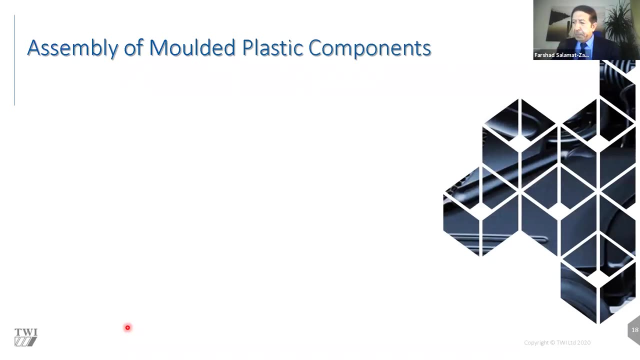 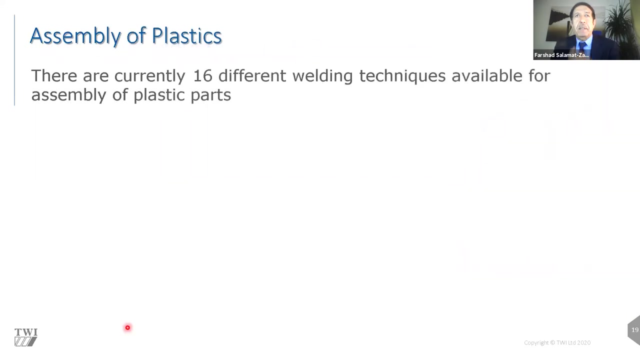 showing the complexity of the design of certain parts and obviously trying to make sure that you know that they're joined around the whole perimeter. it's still so. we looked at the different, different products, different shapes, different sizes. so, as i said, they need to be joined together. so how do we assemble them? 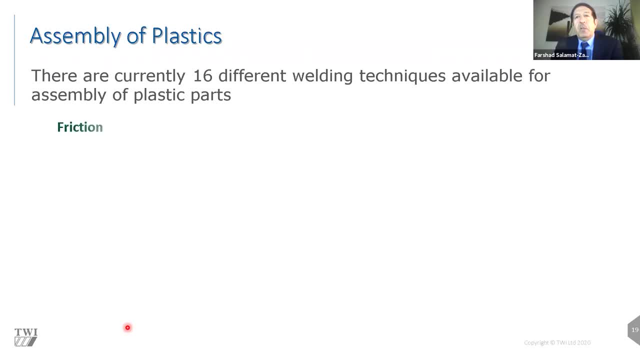 there are. there are 16 different types of welding and joining processes that we need to do for our products and that's several different types of welding that we need to do. actually, some of them are available for for plastics and are. they can be considered or categorized under three categories: friction, direct heat sources or electromagnetic. 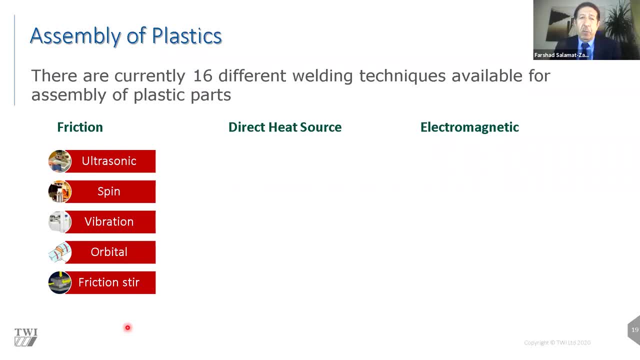 on the friction and we can. we can categorize ultrasonic spin, ultrasonic welding, spin welding, vibration welding, orbital welding welding and also friction, a separate welding, which was one. It could be a heater tool. The heater tool sometimes is called a butt fusion, sometimes called hot plate welding. 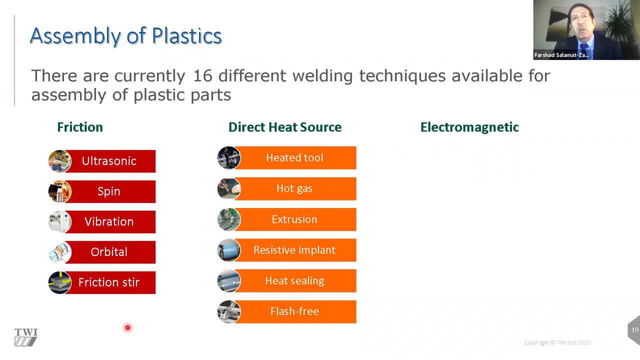 but they are different names for the same technology. So heater tool, hot gas welding, extrusion welding, resistance implant welding, heat sealing and also flash free. And finally, under the electromagnetic category, we have the infrared welding, laser induction welding. 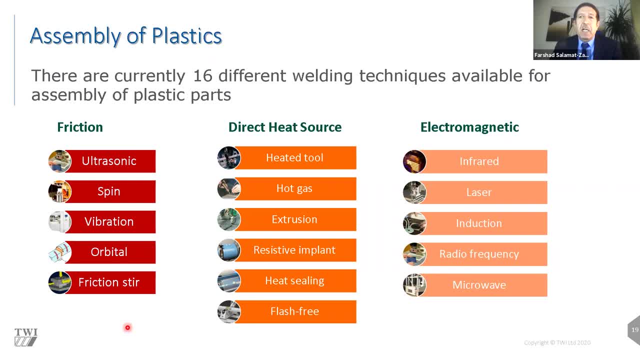 radiofrequency welding, and a more recent addition to the list is microwave welding. So we can see doubt about different welding process welding technologies available. each often will have their own set of tools, set of equipment and set of parameters, And those parameters got to be fine-tuned. 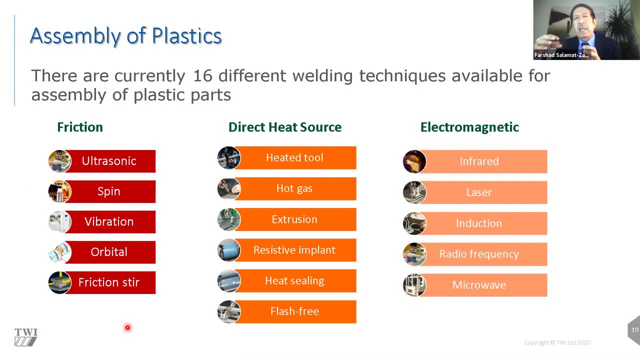 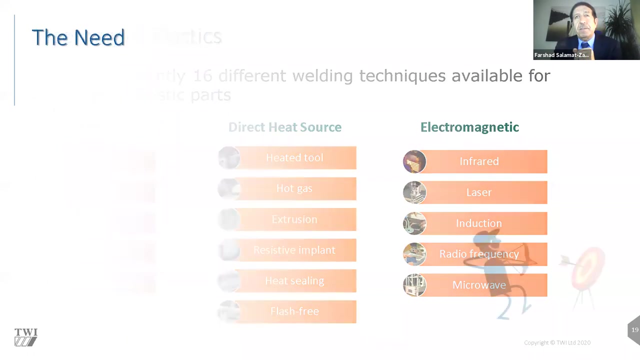 for each application. So there are a lot of other other things which are associated with equipment and welding and joining And, as I said, in terms of the root cause for the analysis, or the same Chicago FM, FMEA, You can see that how these equipment and machineries, they also could be responsible for some of the failures. 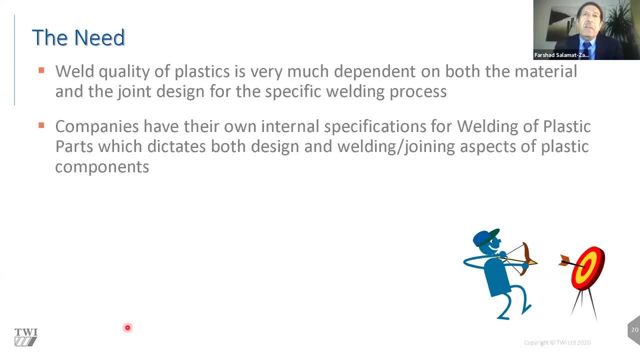 Now, once we weld, once we assemble the parts, the weld quality obviously is critical, How good the weld is. different companies got their own internal procedures for assessing these kind of failures or the quality of the weld And sometimes they look at, they use things like visual inspection occasionally, especially for the containers, for the 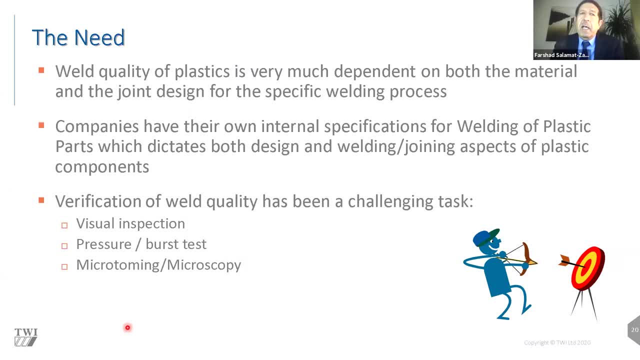 Some of the examples I gave in the previous slide. The container needs. The container needs to be prepared, needs to withhold its welding or is joined under pressure. So pressure tests or leak tests are commonly carried out And also, in terms of the destructive test, microtoming and microscopy can be carried out. 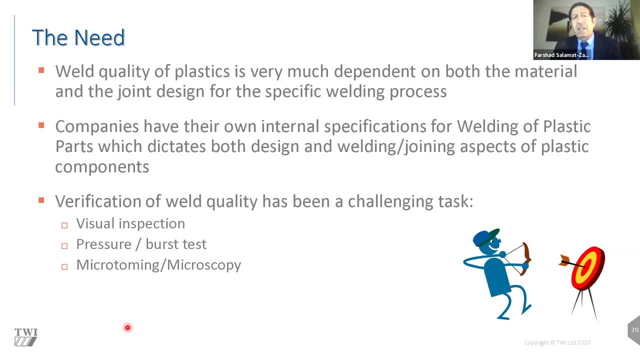 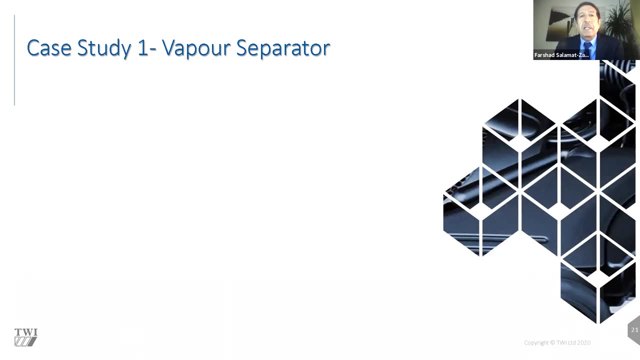 But sometimes this kind of inspection is a bit of hit and miss. Sometimes you can actually very quickly identify it. Sometimes you can spend a lot of time and effort and money and still not identify the root cause. Now, the first Case that I'm going to give is a vapor separator. 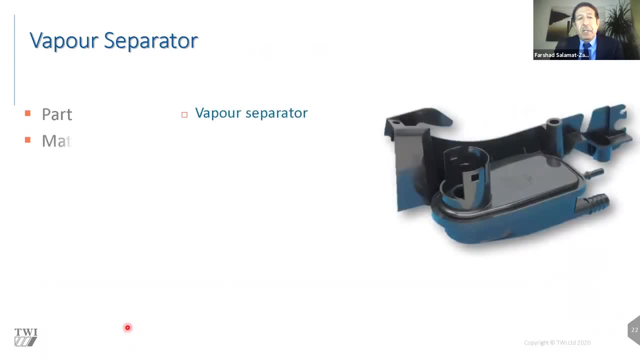 And it is a part that you see in the diagram. Obviously, what you see in the diagram is actually now is assembled part. It's made of two parts. The material is hostaform, which is POM, And the process the way it's been done- both the lid and the cavity of the container at the top. 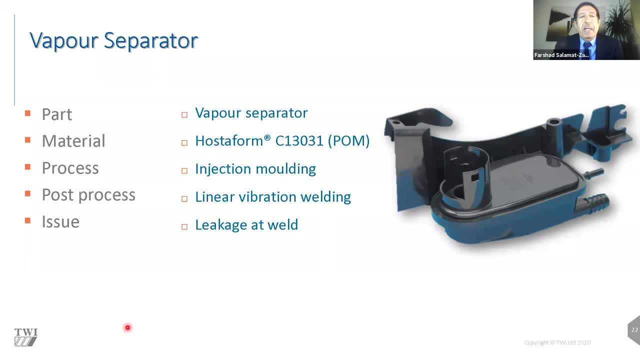 they've been made by injection molding And at the post-processing they were welded or assembled together using linear vibration welding. This is a technology where you vibrate and the material starts to melt due to friction and the heat generated at the interface, And the leakage happens because of failure. 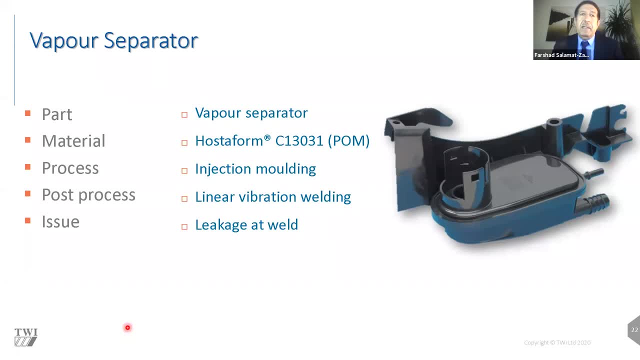 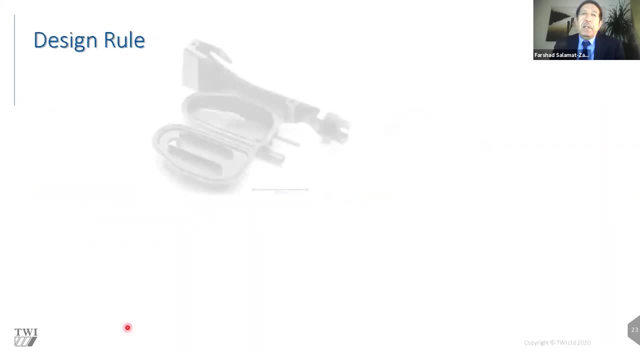 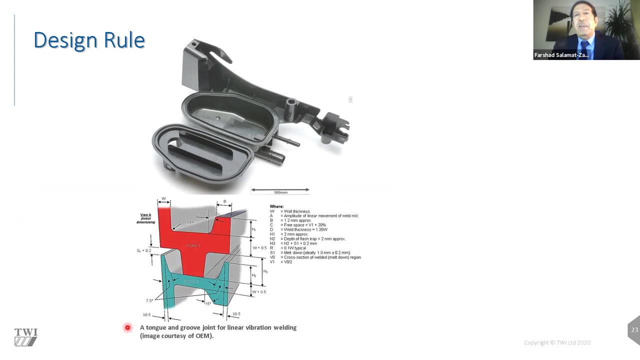 How they assess that. they knew that there is a leakage, So they started doing- They started doing a failure- investigation of that. So, in terms of looking at the component, as I said, this is a two-half component And it's been designed in a way that it's got tongue and groove. 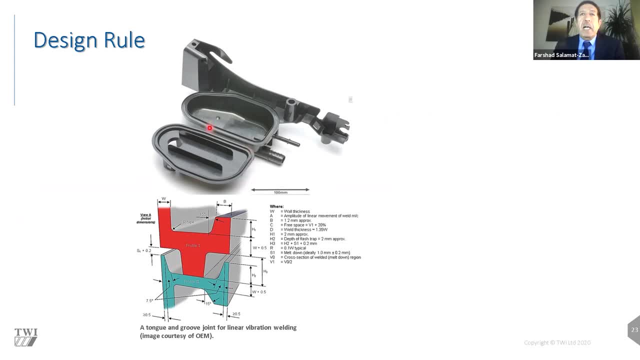 The designer decided that this is going to be a tongue and groove assembly. So on the lid there is something which is a protruded tongue, they call it- And in the cavity in the perimeter there is something like an edge And in the design role, this is the tongue that I'm referring to. 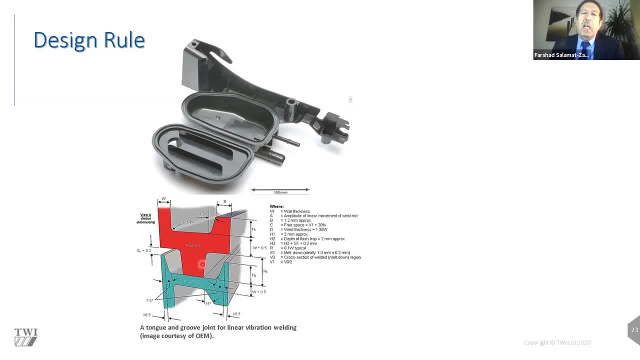 And the edge shape of the cavity. the groove is where the molten material is supposed to be accumulated and collected there. So you can see from the design role: everything is identified, designed and calculated and the measurement is associated with that. 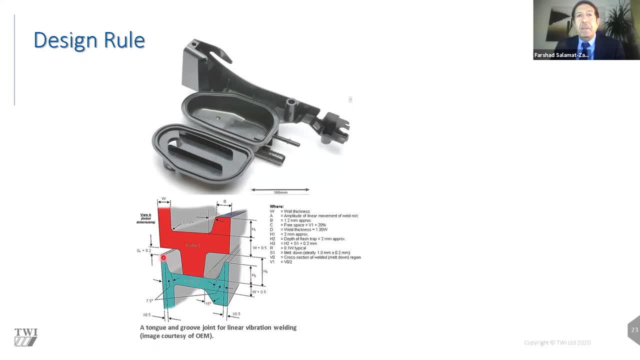 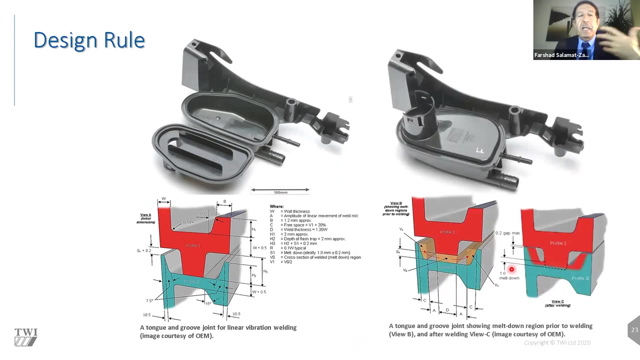 So this- The height of the tongue, the width of it and the gap between the weld gap- all of this has been pre-designed and pre-thought about by the designer. So, once the part is welded, what we need to do? we need to compare it against the design role. 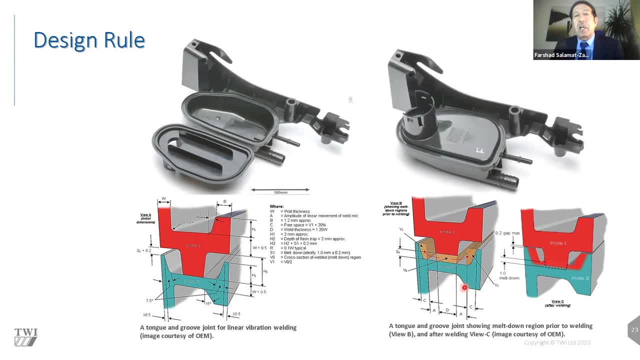 and see whether it actually complies with the design role, with what we started and have it finished up with what is intended. So we need to compare the actual product with the final design role, Final design role, white light and see whether they match. 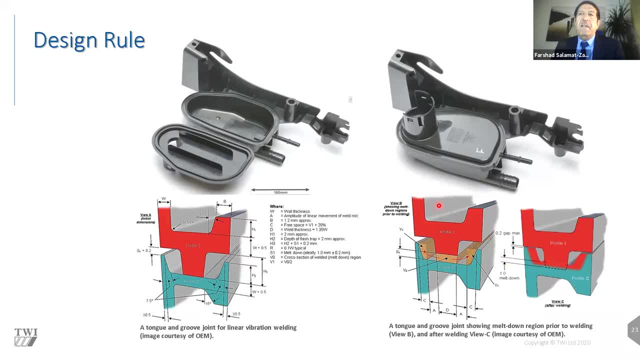 In here we can see the tongue and groove as a mid-process. You can see the tongue and groove is starting to melt so it can be shown by different color And we can see some of that melt is starting to accumulate in the gallery of that edge shape of the cavity. 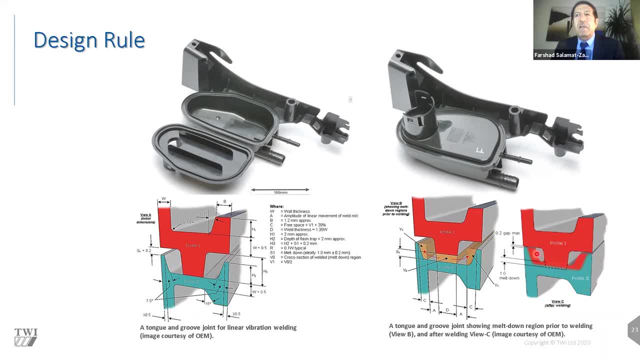 And by the time that the part finishes, you can see there. obviously the tongue has It's white, but it is at the expense of forming a good weld And we can see the weld gap. the weld gap of 0.2 millimeter has been specified, for example, for this particular product. 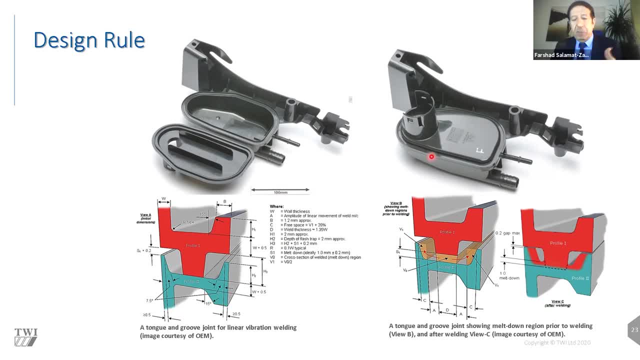 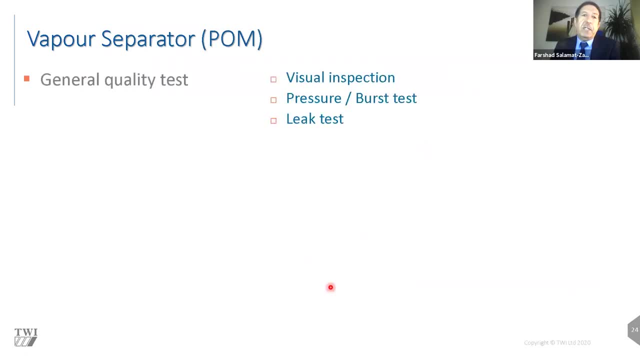 So there is a design rule and there is an end product which we need to compare. So, as I said, generally they carry a visual inspection, So we see the deadly pressure versus or leak test And this particular part in service. it was supposed to withstand three bar of pressure. 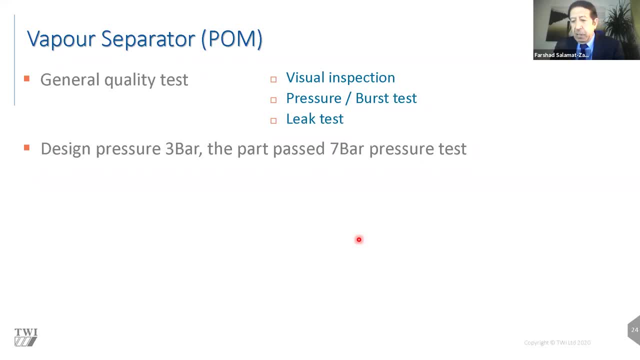 But in testing it passed seven bar of pressure, so it surpasses the design requirement. However, this part failed within the warranty within the first few thousand miles that it's been used. However, it is very important to note that this kind of failure 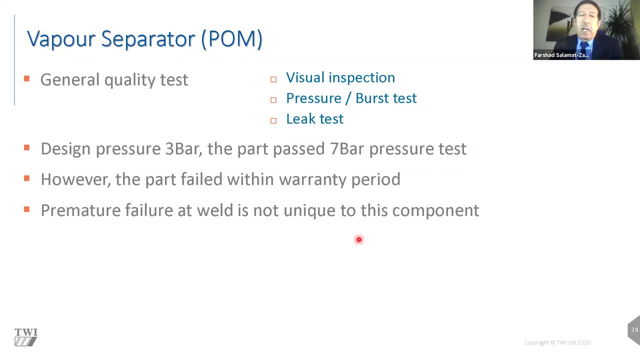 of failure is not common and unique to this part A lot of companies. whether the part is a vacuum cleaner, whether it's a car or something else, failure happens and sometimes, obviously, these kind of failures can cost money and effort to put right. 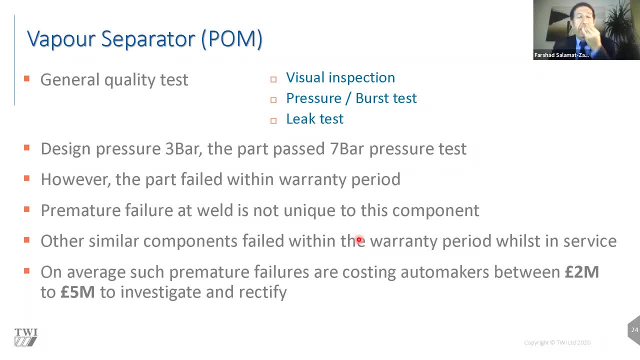 For an automotive company, for example, where they have a lot of different products, the failure, identifying the failure and putting the failure right can cost them something between two to five million pounds annually. So you can appreciate that it obviously has got a great knock-on effect, but worse than the actual cost. 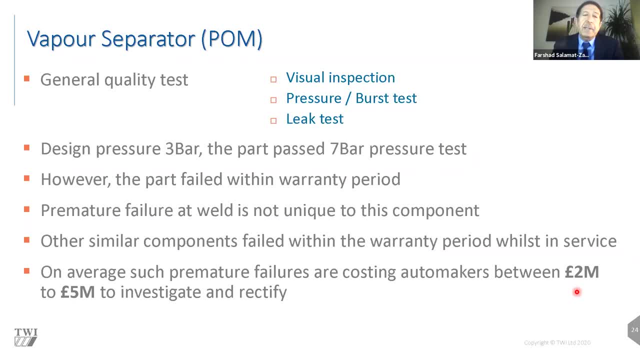 of two to five million is the damage to the brand itself. If, let's say, an automotive company, the brand because of the part that they have which might have been done by tier one supplier, but if the part is failing, nobody would remember the tier one supplier. 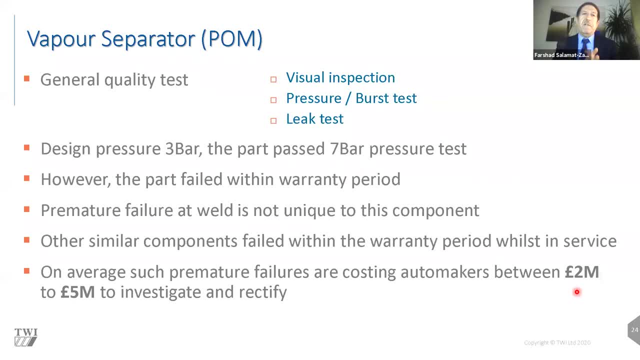 Everybody would remember the brand, the car brand that actually that car failed within the warranty or in the early usage. So the brand will get affected and it gets stained and obviously that's a recovery. Recovering that brand, the tarnished brand, would be time consuming and 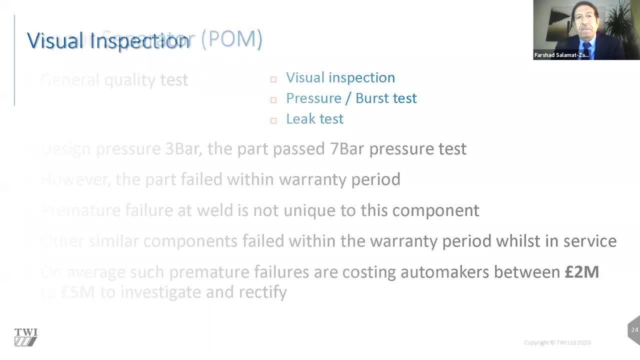 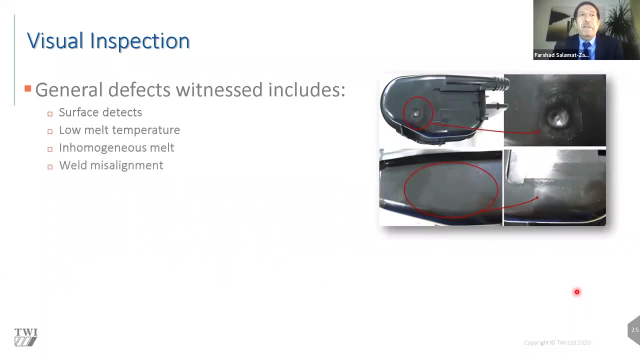 would cost more than the two to five million pound that is stated here. So the best thing is really to avoid that. In terms of visual inspection, what do we look for? We look for surface defects, Sometimes the surface defects. I'll put a couple of pictures there. From the picture you can see. 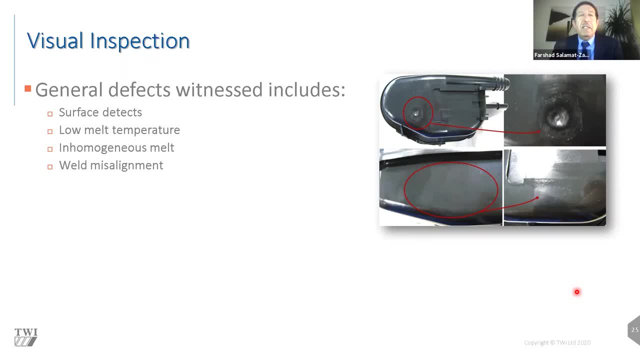 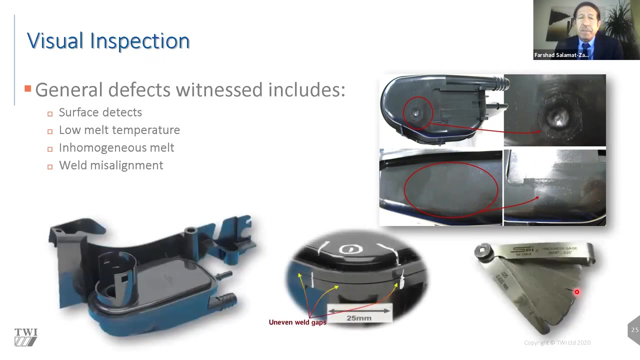 obviously we can see the injection point. we can see low melt temperature phenomena there, we can see a bit of inhomogeneous melting, probably, and we can see a bit of weld misalignment. What do I mean by weld misalignment Is that if you look at the component, the welded component, and just visually go around, 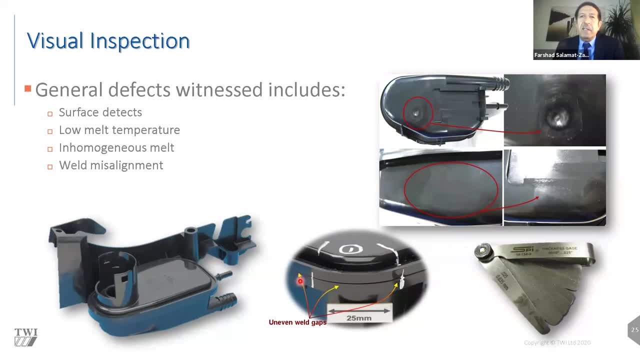 the perimeter and look at the weld gap, we can see inconsistency in the weld gap from at various corners. We can see that the corner is, for example, this gap is increasing And, as I said in my earlier slide, where I showed the design rule and I showed it and I 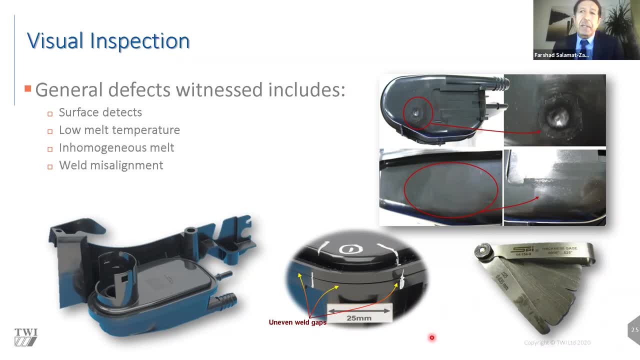 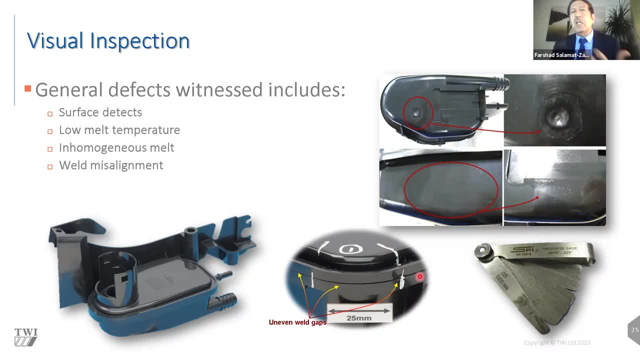 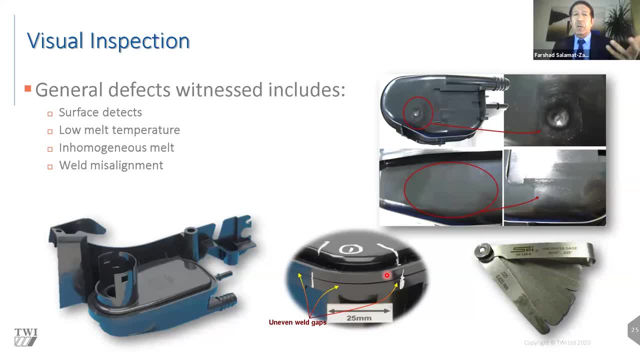 and either it's scrapped apart completely or you know, obviously, if it's faulty, And in order to make sure that we are consistent and we don't rely on different individuals and their eyesight to see whether this is a 0.2 millimeter or not. 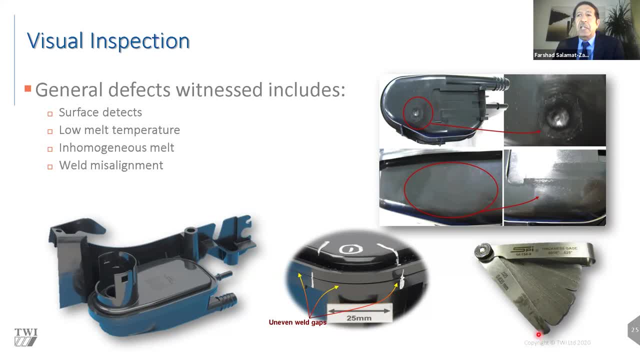 they can very simply use a filler gauge, whereby each of these blades got different thicknesses, and these are all pre-standard. You can buy them in an imperial unit, or they can be SI. And then what you do? you can choose a 0.2 millimeter gauge and take it around. 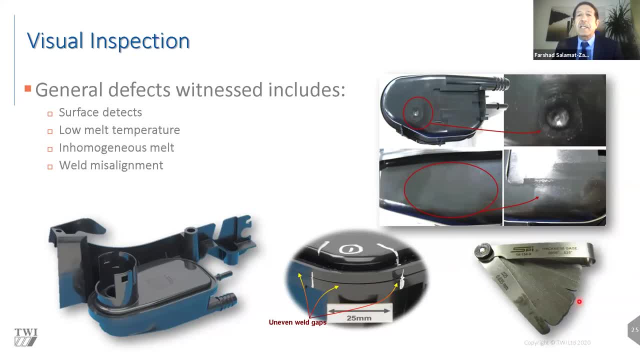 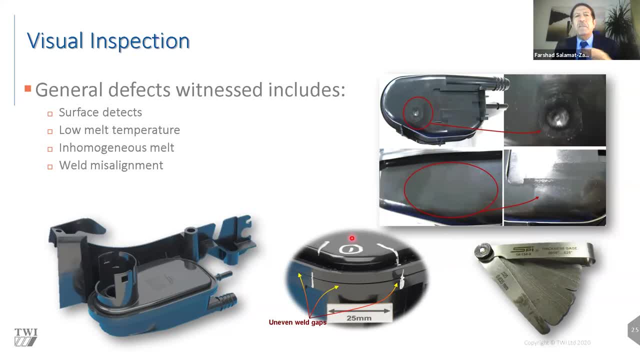 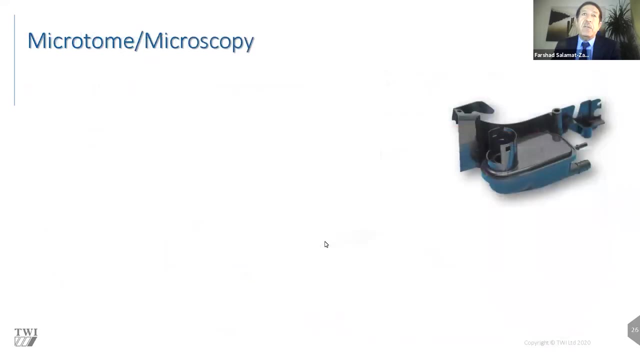 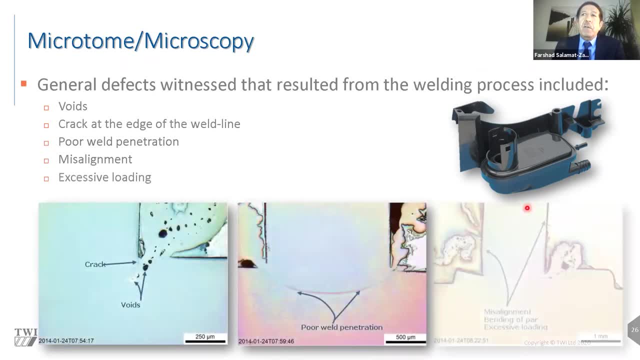 Also, the use of rod geschmack may be forceful in that regard. uh, you can what you do, you can. you can. you can cut the part, cut the component into cross section and look at this cross section under the microscope. but that's a bit of the hit and miss, are you? 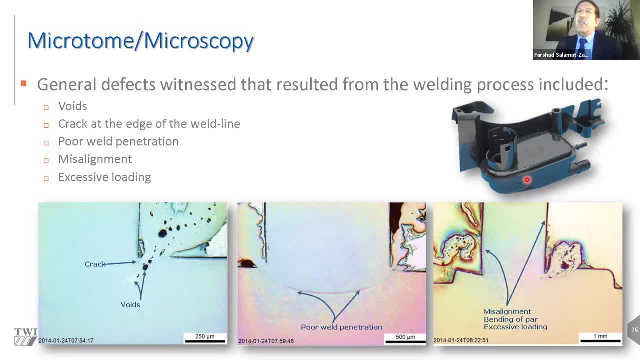 actually looking at the part that might be of concern, or you just look at the part that might be actually good, good, well, however, what? what i've done in this case? i've taken, uh, this, uh, i think, a number of corner corners and i looked at the various corners of this, uh, of this motor part. 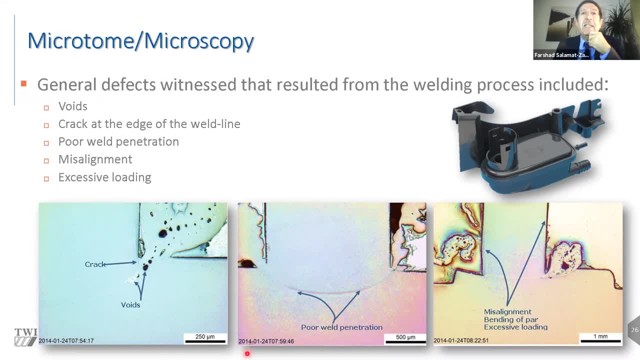 and from from the micrographs that i presented here, we can see, we can see some issues. we can see, for example, crack at the belt, so we can see the crack is running down here, or we can see a lot of voids or blisters. this could be. this, for example, could be: 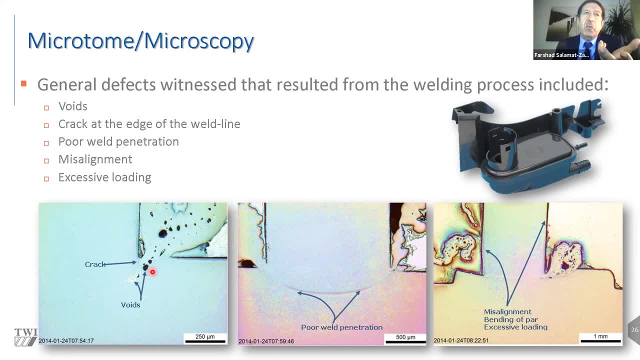 due to the water moisture within the component- maybe the component was not pretty dried before welding uh- and or or the loss of, you know, volatile, volatile compounds or other additives that is causing this uh during the heating process. but obviously what you can see, the voids are. 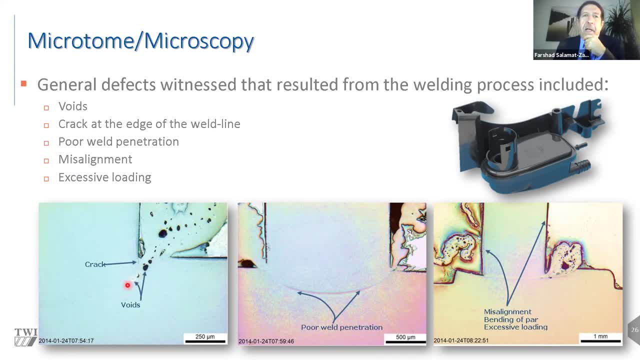 sitting at the at the foot of the well and this uh, obviously if, if, due to poor loading or pressure, you can see that this can start and i can start from there and can propagate. and you've got a very, very weak uh interface here compared to, for example, to somewhere. 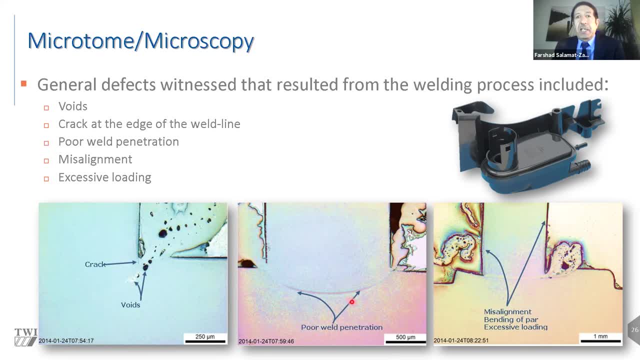 that i'm pointing out here, other issues. you can see poor weld penetration- you can again that's with microscopy, that's quite evident- or you can see misalignment and buckling. so there is a lot of overloading on one on one part, and rather than this- the tongue to be straight- here we can see: 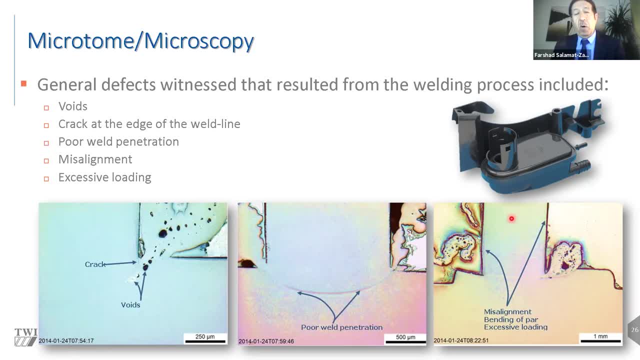 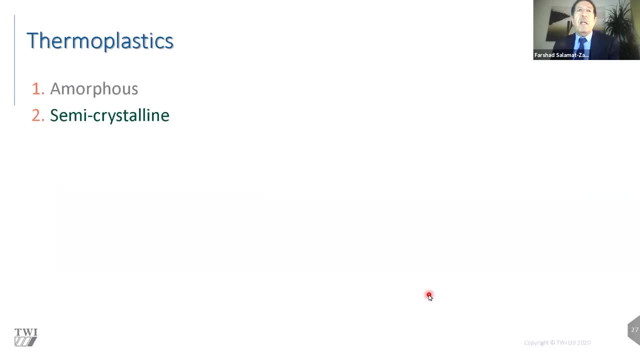 the, the bending, so we can see that there is a bit, there is a lot of overloading on the component. microscopy is useful. however, just just to touch about, why do? why do we get this kind of changes in the product during the welding process? i need to reflect back on on the. 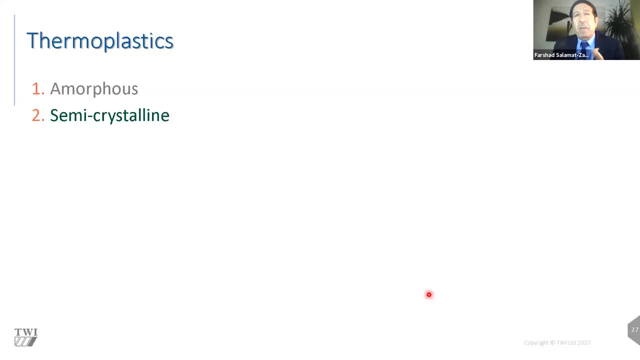 the thermoplastics which these these components are made of. thermoplastics as a, as a simple term, they can be either amorphous material or semi-crystalline, amorphous being basically the polymeric molecular chains which are all randomly uh spread, whereas the semi-crystalline they have both, both the the random structure of the of the 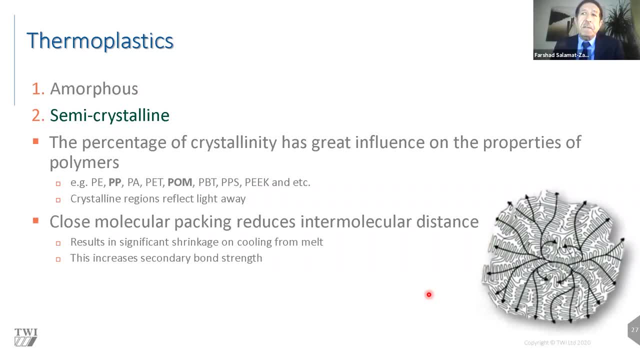 morphos, but they also got a highly ordered crystalline region, which is, which is these areas that i am pointing at. basically, this is, molecular change is folding back on itself and they create a 3d, a sterolite, and and that's what? uh, from the crystalline region of a, of a crystal. 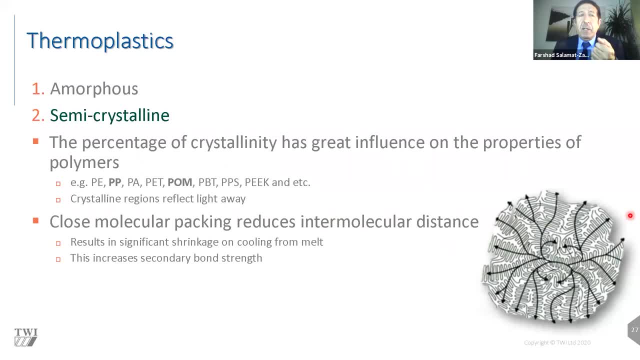 so i've given examples of some of the semi-crystalline materials here and i'm also. the point i need to make is that, obviously, as the material starts to crystallize during the melt, all these molecules are are randomly moving around and as as they start to cool down, these 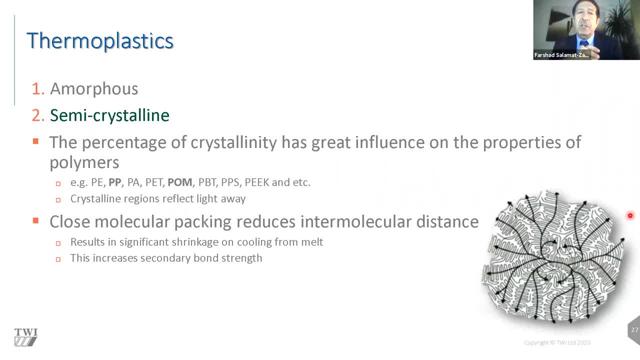 these molecular changes start to fall back, especially the crystalline material. they start to fall back and as they're falling back, we can, we can understand, we can imagine that the material is actually or the part is actually shrinking because the all, every molecules from long chain, molecules from different angles, are gradually retreating because of this folding. 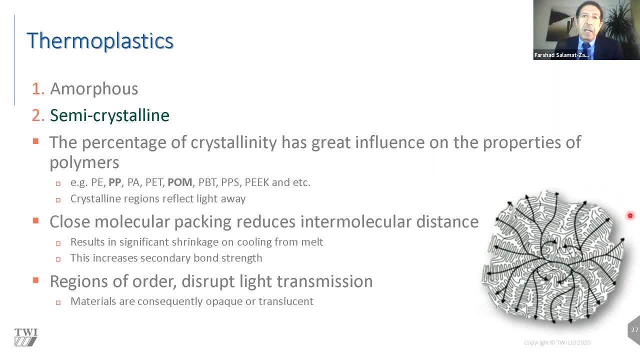 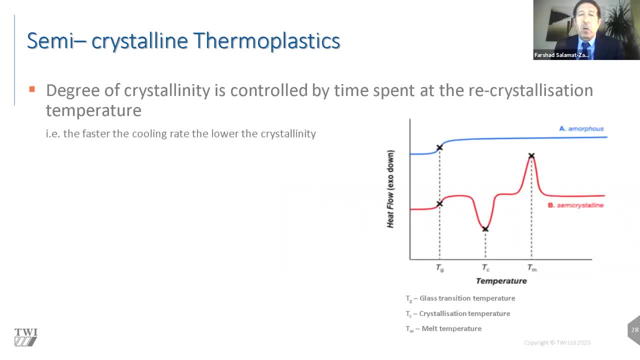 folding back mechanism. so just just touching on the of the semi-crystallinity a bit more. basically, what we have here? we have a, a dsc, which is the conventional scanning calorimeter plot of an amorphous material in blue. uh, here it is against a semi-crystalline in red. now we can see that as the as we start heating. 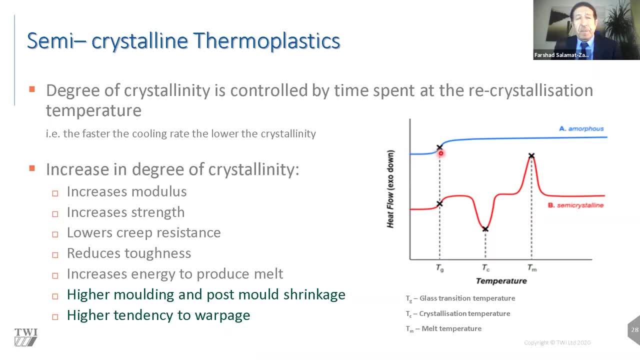 the material from the solid. the material starts to get close to the last transition temperature and by definition it is a range of temperature at which the molecular motion starts to happen. so the molecule starts to become mobile. so the material from solid is becoming a bit viscoelastic. 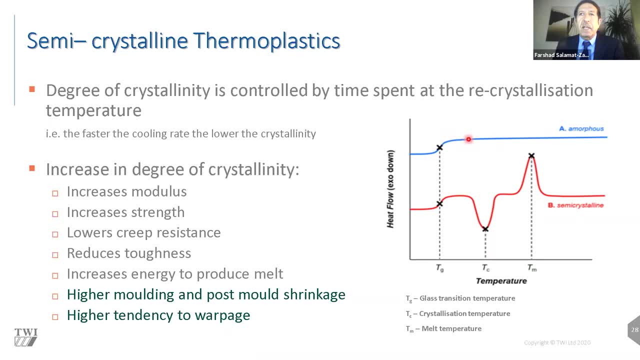 and for amorphous material. once that is passed after there then you get molecular motions. the whole material in semi-crystalline is different because what happens initially, you do go through this phase of glass transition. so some of the some of the molecular changes start to become mobile. 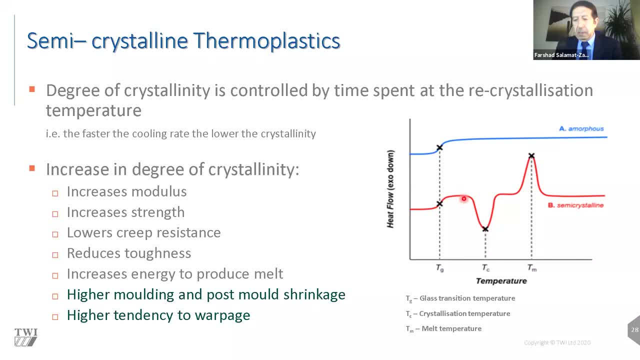 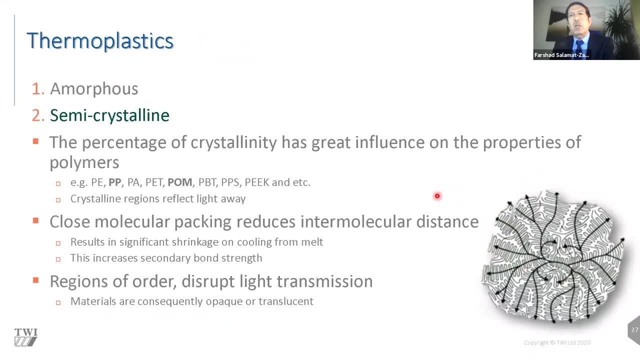 but? but we get to this. if i go revert back to the previous slide, if, if you look at this, this diagram, so once the initial random random molecule started to become mobilized, then we get to this more compact, rigid structure of semi-crystalline. and, going back to this slide, this is this region. 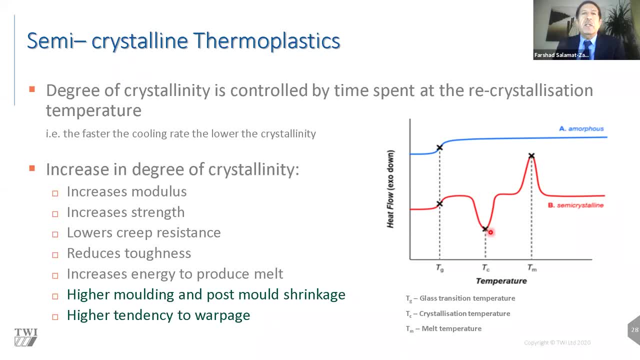 so now, in order to to start making those regions mobile, we need to apply more heat. so we go through the, the crystalline region starts to heat up and obviously starts to absorb the heat and become more mobile, and then we eventually get to the uh, to the melt temperature of the. 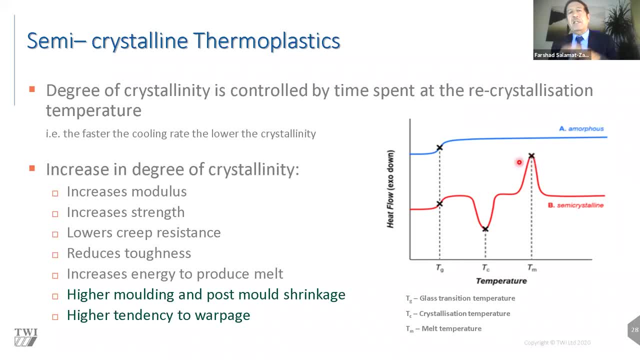 material, after which the both the semi-crystalline region and the amorphous region are fully mobile and the material can actually move around. now the reason I'm displaying this is to come back to here and explain to you the advantages of this principle. disadvantages of increasing the degree of crystallinity. well, by increasing the degree, 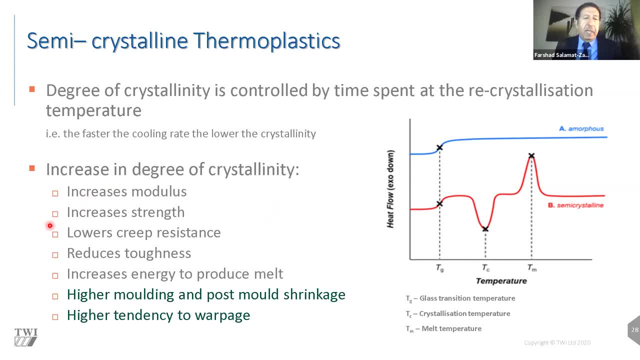 of crystallinity. you can increase the modulus, you can increase the, you can increase the, the strength and the uh of the material. but there's always compensation. uh, you have. there's a compromise. so the compromise here is that that that is at the expense of the uh. it lowers the creep resistance. 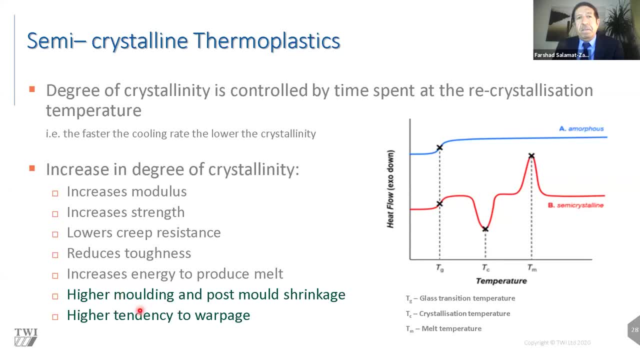 and also it reduces their toughness. but because of this shrink, because of this, uh, when we come back from the molten material to the, to the, the solid materials, then we are cooling down as a, as a molecular change, as i explained earlier, it starts to fall back. 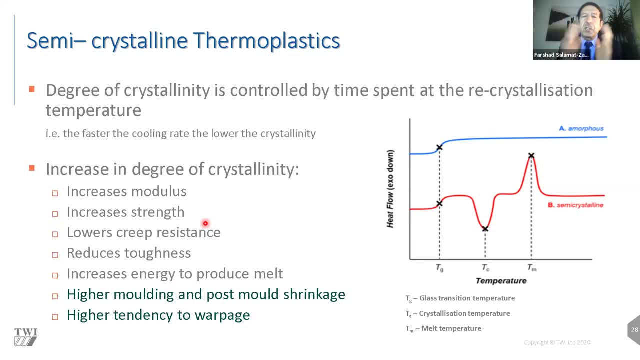 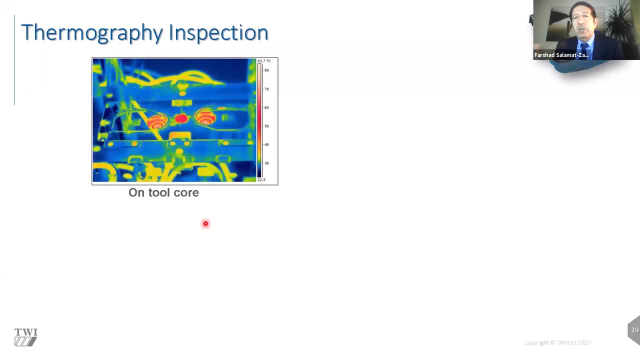 to. we do get this uh mold shrink so that the part starts to shrink, and as they shrink, if the shrinkage is not uniform, then you start to get a bit of warpage as well, and what we see in one of the one of the uh images that we saw earlier was due to the warpage. the reason that 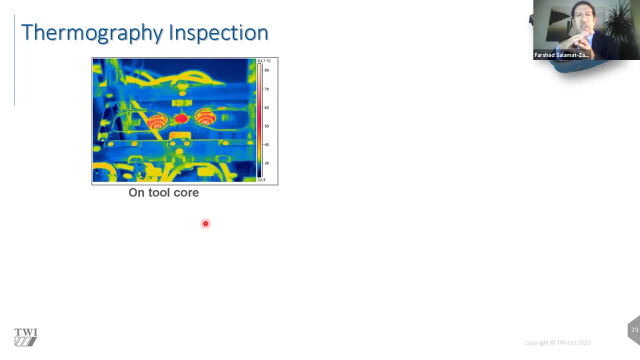 the lid. the lid of the lid was was a special uh was slightly at a different angle and we had different valve gaps around the perimeter was due to warpage. let me get to that a bit more. so how do we assess that with product? one way to do it is to use a thermography inspection. 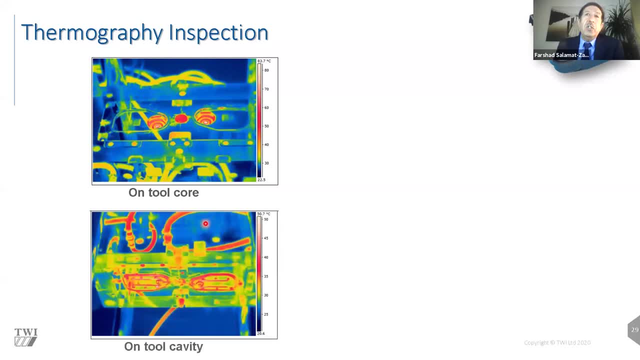 so thereby, in this case, we are looking at the tool during the injection molding. so we're looking at the at the cavity and the lid of the part. we can see the cold part. obviously there are a lot of water channels going through here. we can see the copper and we can see the regions which are pretty. 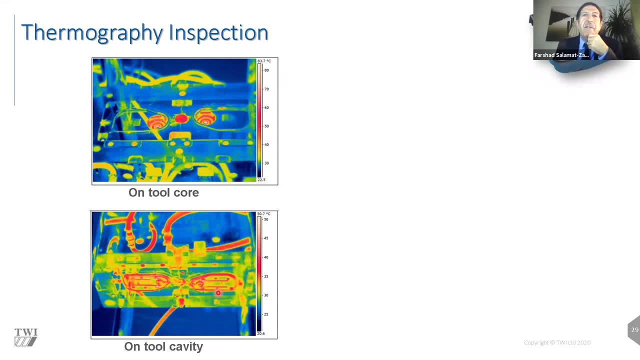 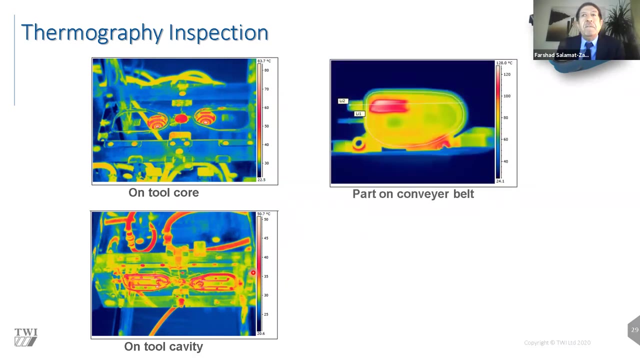 hot in the tool. so, and this is the cavity, and we can see all the pipe work that goes and feeds that. but this is the on the tool itself. but what will happen with the part when it is ejected from the, from the injection molding tool? looking at the cavity, this is the. 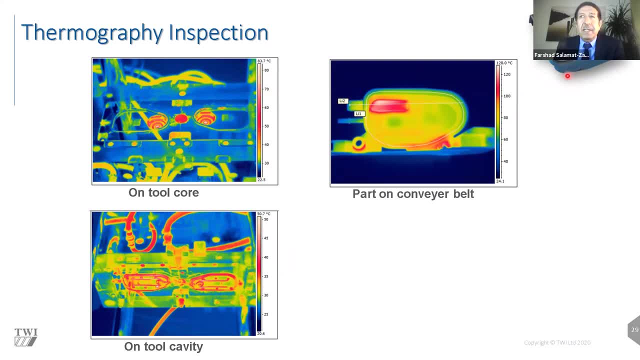 the, the bottom part of this. i call it cavity or the base. this is sitting on the conveyor belt. the thermograph shows hot zones in various parts of this part. these hot zones, what they do? they allow the crystallinity to continue. so the crystalline keeps continuing, so the degree. 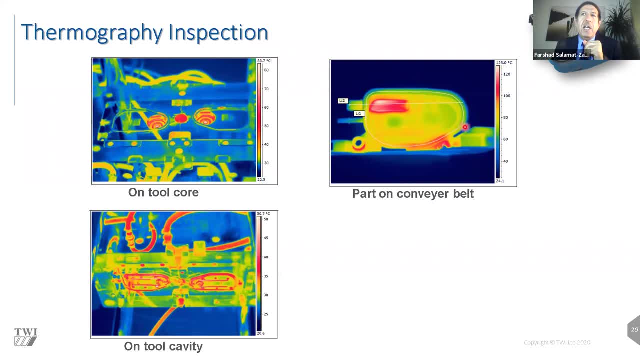 of crystallinity will not be uniform in the area which is cold compared to the area which is, which remains hot. so if you want to have a consistent degree of crystallinity, the whole product got to be cooled down in a specified manner so that you end up with a uniform degree of crystallinity across their. 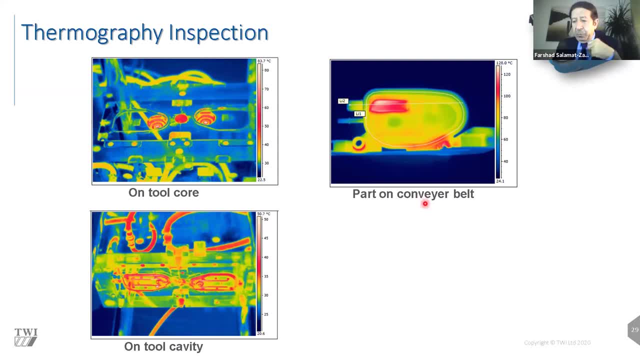 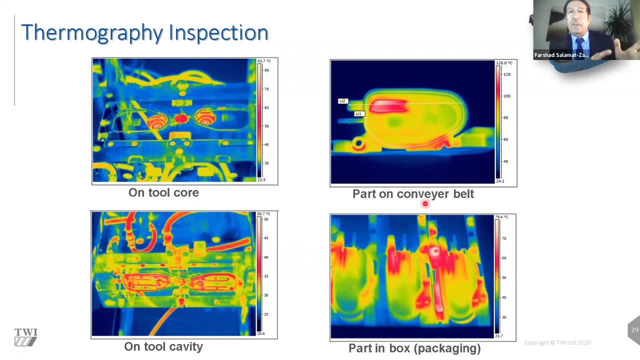 product. otherwise you end up with hot spots. and to make it worse this, these components are then stacked up in a, in a cardboard boxes or whatever, in order to be dispatched to a another company or another, another department where they do the actual welding. so these hot components you can see, 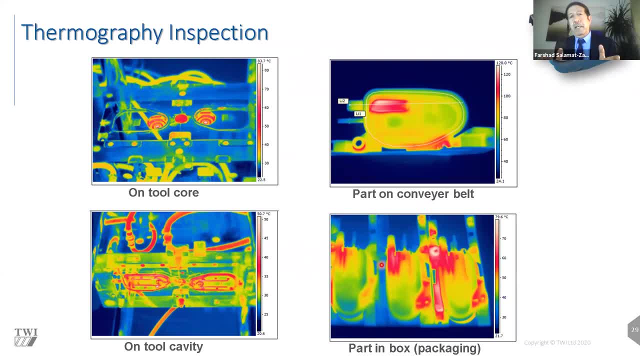 hot spots on a number of these cavities. they sit in a in a cardboard box and the heat remains there and there is no way of cooling it and and this degree of crystallinity keeps rising and rising and rising. so, but these are. this is critical, that that's an indication that obviously something 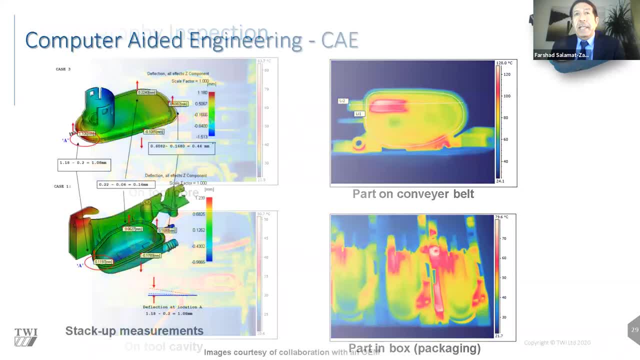 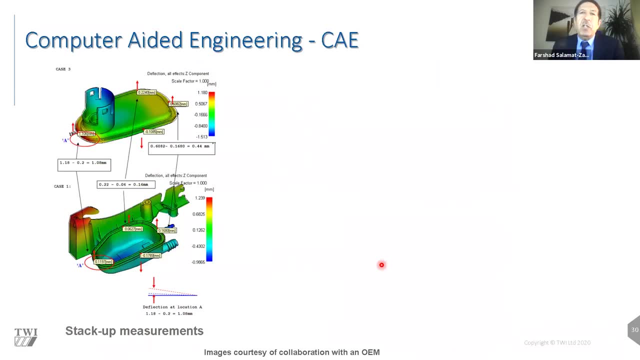 needs to be done here. another technique is computer aided engineering, whereby we can we can design and, considering all the material parameters, you can actually see, you can simulate that, the shrinkage that i talked about. so, as the, as the component is made, you will get this shrinkage and you can see how the lid and the 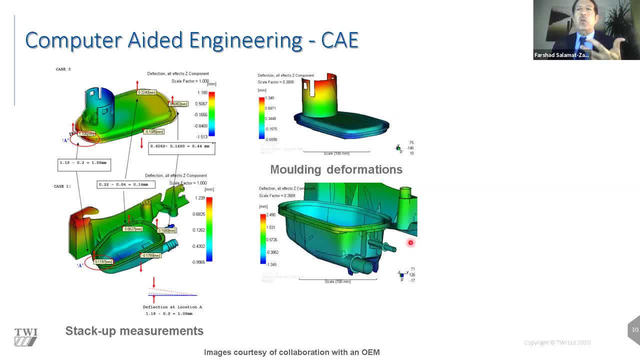 component is shrinking but again, this is based- this will be based on the uniform shrinkage. again, we can see here we can see the hot zones that that might be created. so if you are aware of it, we should find a way of resolving it before going to the actual product. 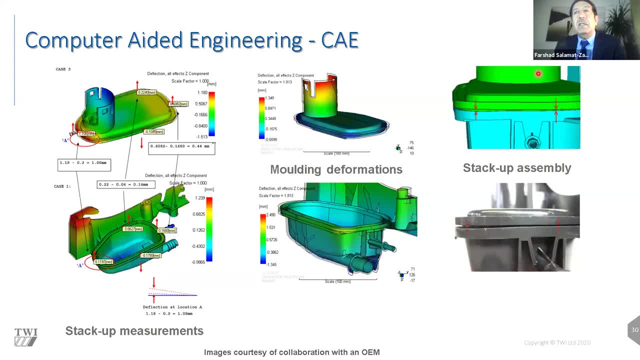 so we can see. we can see the influences. so the simulation cae shows us that because of this warpage and shrinkage, we might get discontinued and we might get, we might get a poor weld gap and we can actually see it in the product. as i said, it's obviously. this is the worst case scenario. 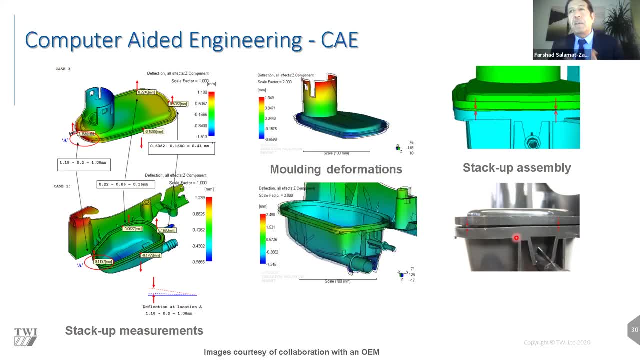 very exaggerated, poor, but a poor example. but sometimes a product is better than this and passes the test and goes into a and goes and gets assembled into a, into a car or or another product, but then we find out that very soon you will have a premature failure because certain things 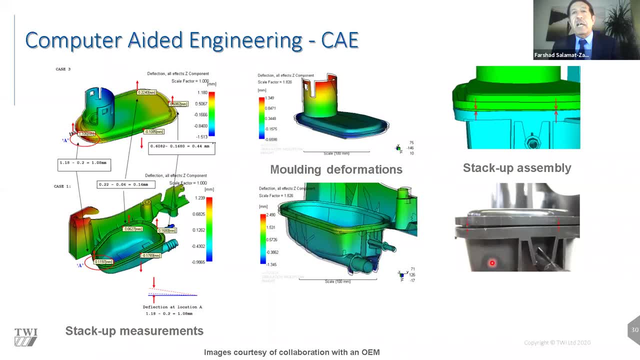 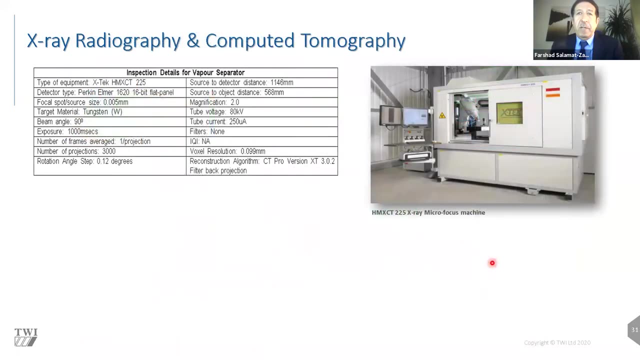 wasn't done right and we come to that again later. so this was another technique, the engineering- and tell us and can warn us of the consequence of some of the things we're going to see. okay, another technique which i do, quite a i don't know eight, ten years ago, i introduced a couple of 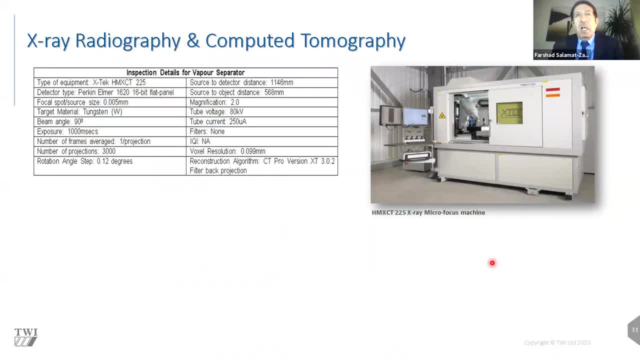 oems in terms of inspection is the use of x-ray radiography and computer tomography, whereby the same product is x-rayed. so you build up about thousands of 2d images of the product and then the computer tomography side of it. it brings all these 2d images and makes it into a conversed into a 3d object. 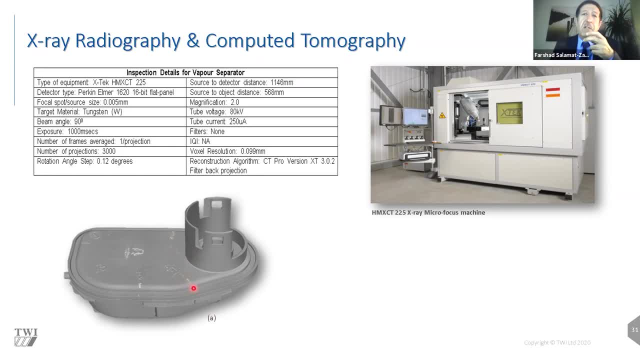 as you can see in here. so what? what i've done? obviously we mark different corners with the number, so we can see the numbering here, but we can see the component and more detail once it is made into a 3d component. as you see, i can actually cut, cut across this. 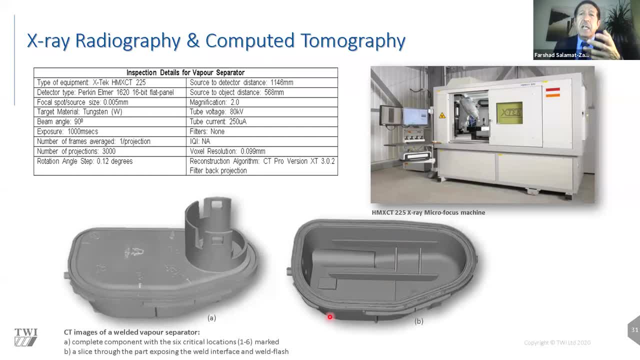 at any position i want. in this case i moved halfway down, just around where the lid and the and the cavity or the base is, and i can. i can look at the interface of the weld. this is non-destructive, i have to stress on that, and we can see the, the weld flash in certain area. 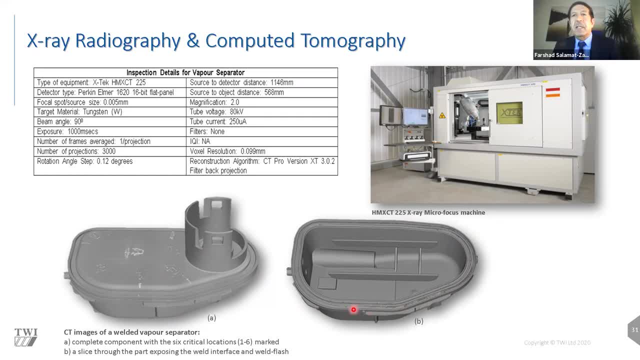 the excess welding as a result of that on melting, but we can see the absence of that in other areas. So just by looking at that, you can see inconsistent welding in certain parts compared to other parts. So there's an inconsistency in terms of how the two parts are welded together. 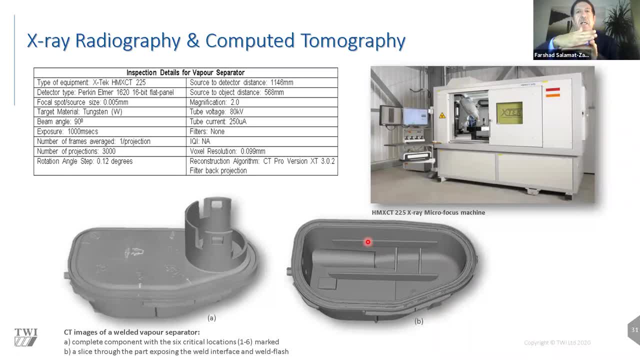 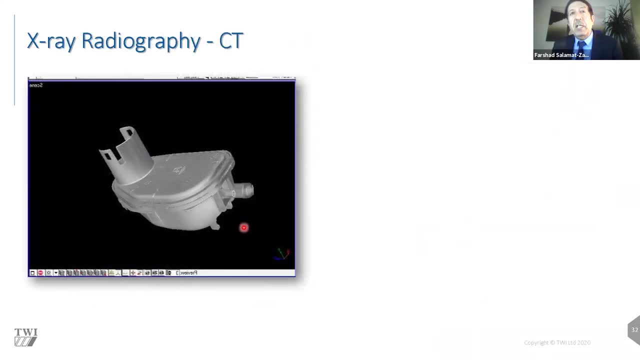 Now, it could be, as I said, it could be due to that warpage of the lid or the base, but we can see it here, And another thing we can do is that we can actually walk through the product like an MRI of the body that hospitals carry out. 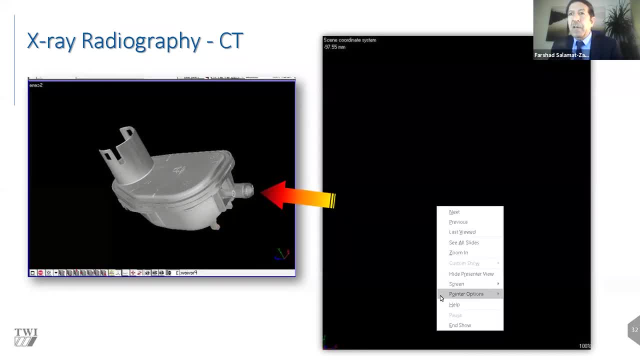 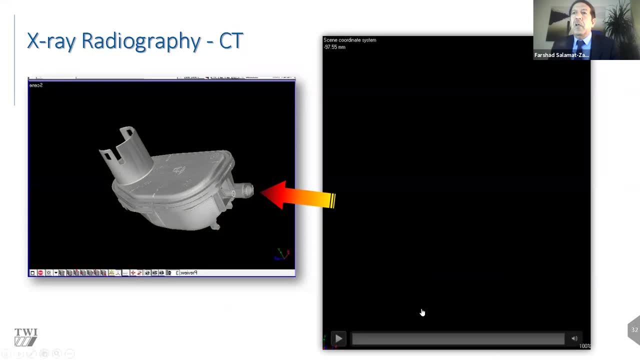 If I just walk through this for you and Okay, so this is a video of it. So we are at the nozzle end. now We'll be gradually walking through And we are reaching to the first side wall and we can see the weld at this area. 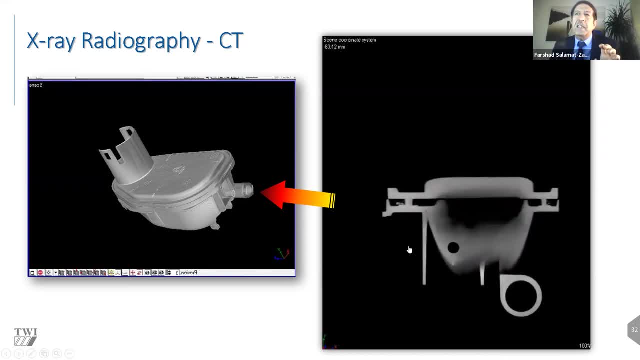 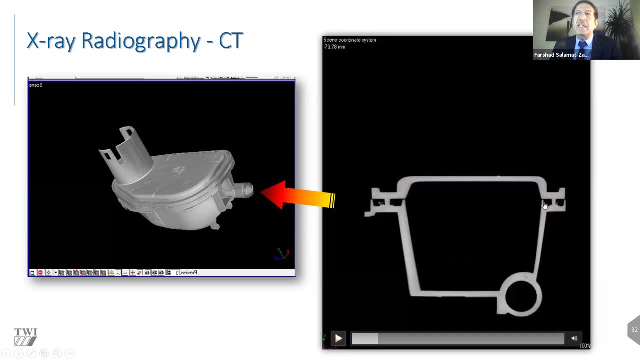 Now we are gradually walking in, Now we are getting into the cavity, into the chamber. Now we have- if I pose here we can see we have a distinct right side and left side, which relate to that side and this side, now right and left. 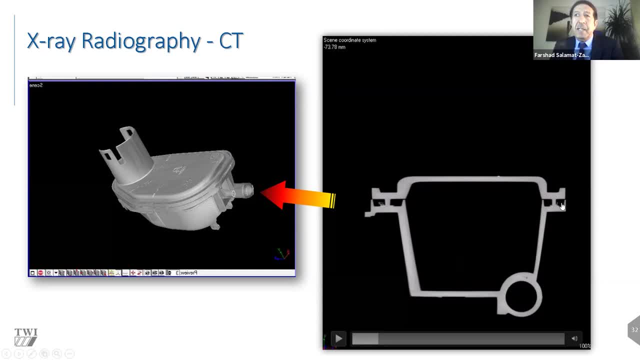 And we can see the tongue and groove and we can see flickers of a weld flash in certain area, certain area and other things we can see. we can see certain voids. as we go through this video, you can- uh, i'd like you to pay attention to certain areas around here where you see different voids. 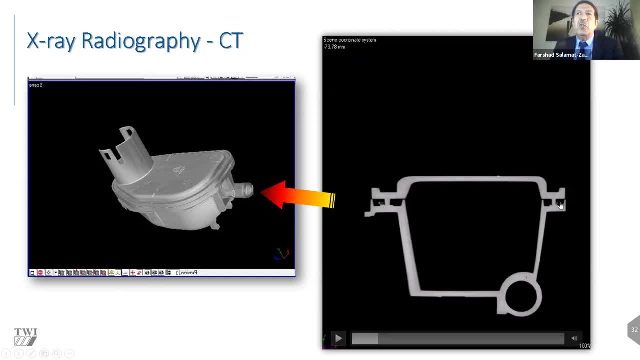 and also, as we walk through, you can just see how much weld we are getting in these galleries. remember from the design rule these galleries got to by the end of it they got to be pretty, pretty, pretty filled up with a molten material. if you continue again, i just as i said, i i put. 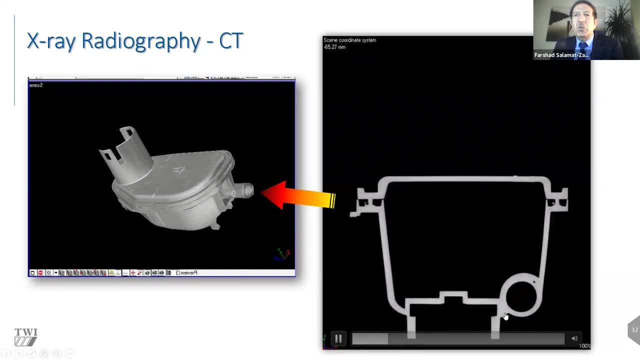 my cursor around where the where the voids are, just to show you that what other things we are seeing as we are inspecting this and we can see a still relatively poor quality of welding. we're not getting any any substantial weld flash in this, in these galleries either. 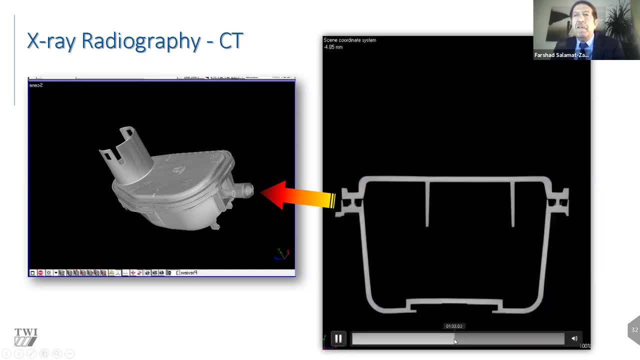 and it's just because of the, the quality of weld flash, the result. if we look at the this, this is not enough. so we are continuing here, we are still looking at the side and we are still moving forward. if i go to halfway and we're getting now to roughly where the 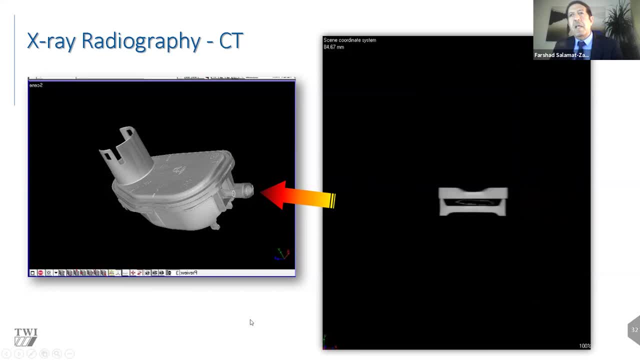 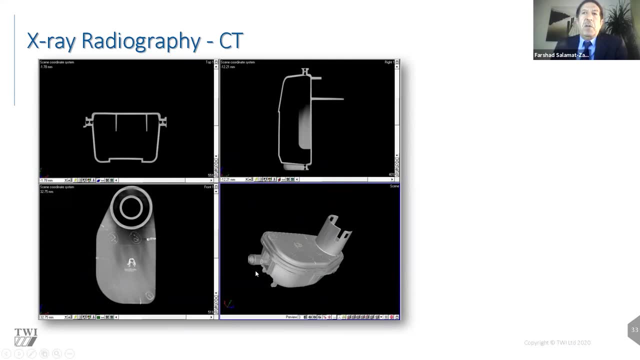 whether what this- the name called chimney is. uh, looks like the chimney, so we can see again. if i pause here again flicker of flicker of weld flash and not enough. basically, this is a part. we can rotate it and we can look at different view of it. we can look at: 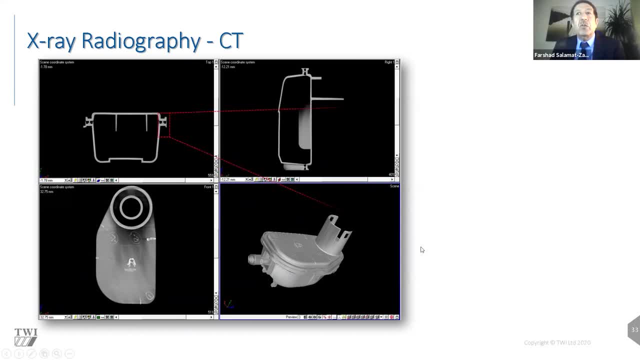 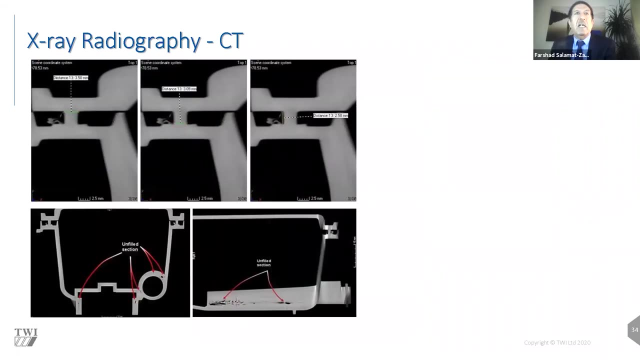 top view, end view, side view, and we can start to scrutinize this and zoom in and try to look at the weld, the tongue and groove, and look at the weld flash and and assess certain, certain information about that. and how do we do that? as i said earlier, we can start measuring that using the software we 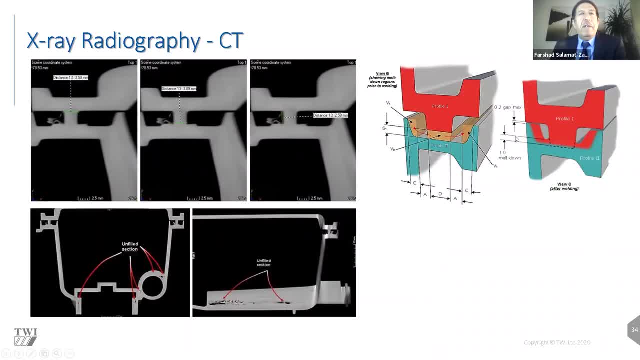 can measure various features of this valve and we can compare it against the design rule that we we stated at the beginning. this is something that the designer has spent quite substantial time in designing and getting it. right now, we need to know whether the at the end, at the end of the uh, at the end, when the product is actually assembled. 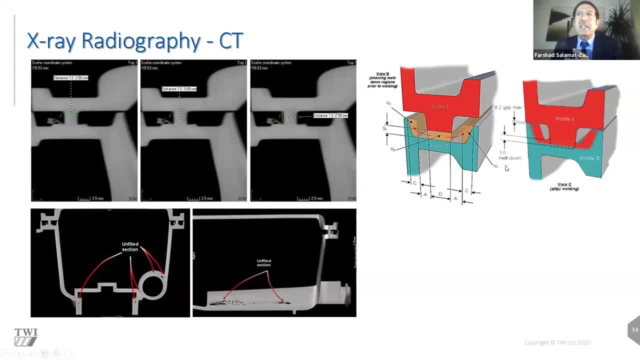 in injection, molded, understand, welded and assembled? does it meet the criteria so we can compare the height of the height of the time, the volume of the production event in a drawing, каких, and how the technology is and how it works with mr? i will let dr lavitt wrap this up. 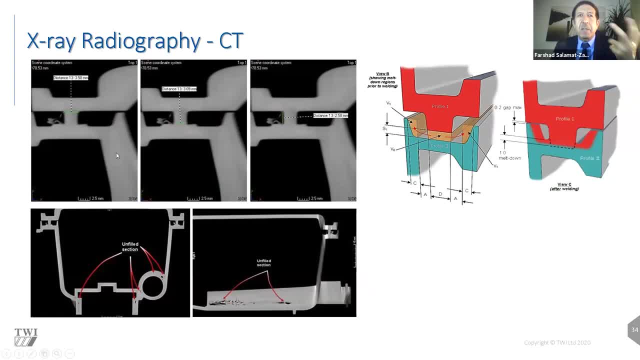 the width of the base and all the other parameters, against the design rule. But what is more, we can also see that the X-ray CT is showing us a lot of voids within the component, especially in the thick section, whereby, due to the retention of thermal heat, 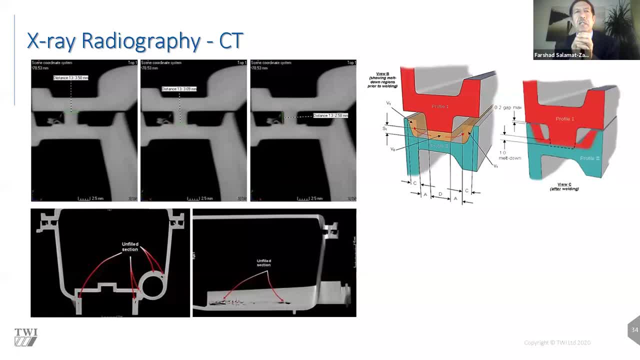 that I talked to you about, because the material is, the heat stays there for a long time, so you get a lot of shrinkage. So the material is shrinking. If you've got a thick section again, you can get shrinkage internally. 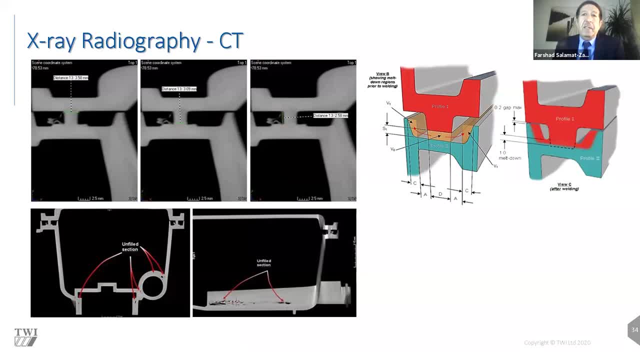 which leads to the void, Or it could be other matters, other scenarios, such as the material has got too much moisture in it and it wasn't pre-dried properly, and then the moisture in the thicker section they show themselves worse, But we didn't see any moisture on the surface. 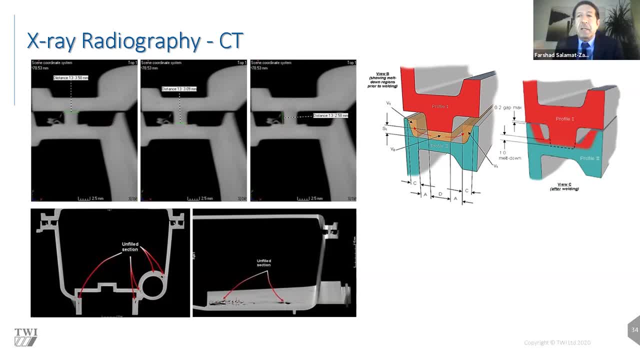 The surface of our clean-off blisters. but the surface of our clean-off blisters is very more internal, So, but the X-ray showed this to us. So now that this component is black, we cannot see. it's not transparent or translucent. 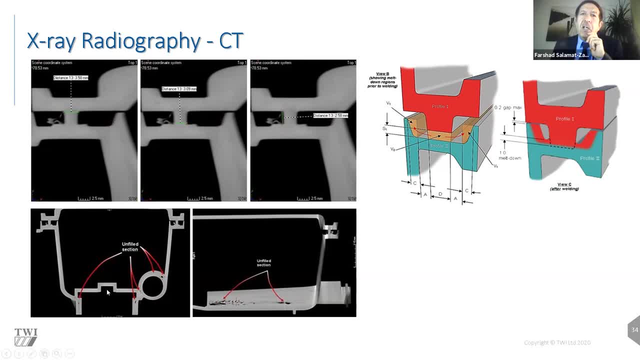 we cannot see it, But by having a loss of wall thickness that means that this material will not be able to sustain the same pressure as a material which is fully solid. But there is less material here, so there is more chance of this failing. 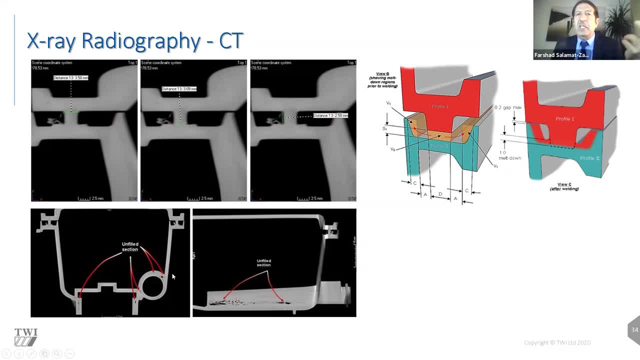 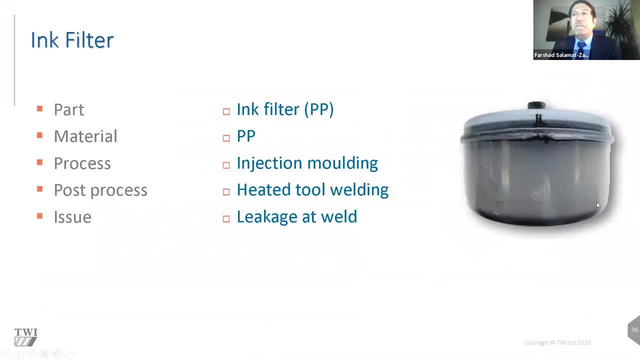 of the failure might happen at the world which is slightly weaker than that. But if the world was of good quality, you might get failure somewhere else where there's a lot of void within the material. So something to be aware of Now. the second case study is an ink filter. 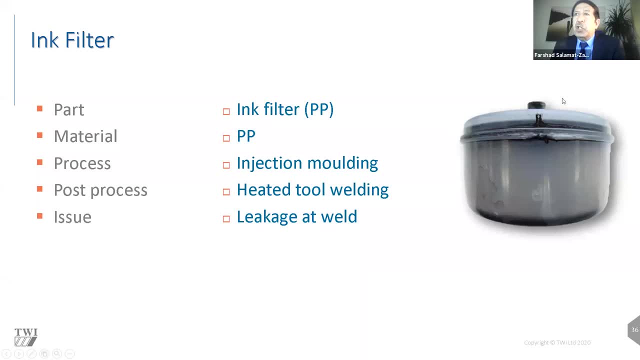 Basically, in this case the material is polypropylene. It's made of a chamber and a lid and certain sub-component It was made by injection molding, but this time it was, it wasn't made of polypropylene. It wasn't welded by the linear fraction. 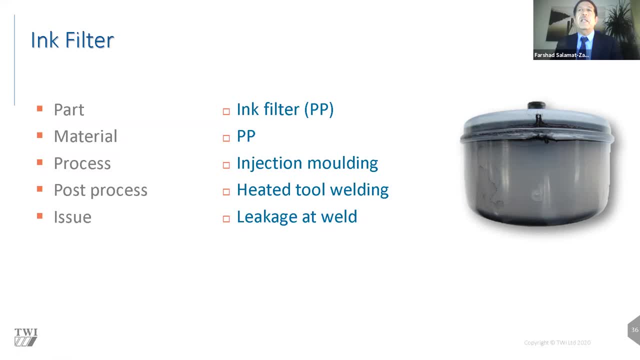 It was welded by heated pool welding or hot plate welding, where both parts gets heated with a heater pattern and then they brought together and then under pressure or distance for set time and they get welded. Obviously we can see a bit of the pool quality. 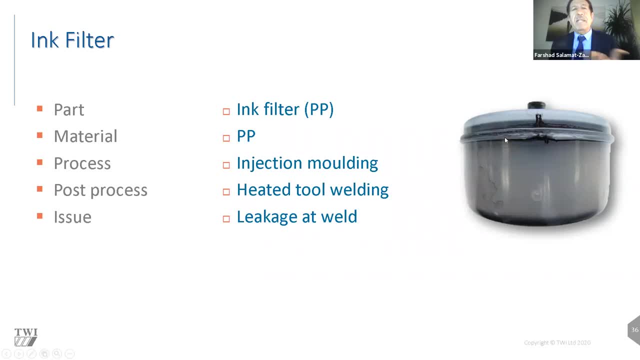 of the weld on the outside, but this is probably the aesthetic of this was not critical for the applications because it sits inside a printer somewhere, So but we can see there are some territory sign up. Maybe the welding is not great. Again, the issue was leakage at the weld. 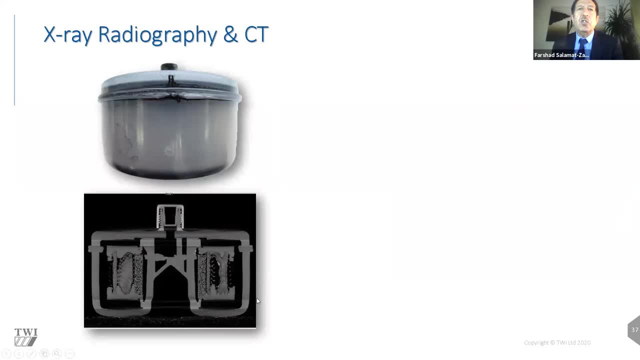 So XCT X-ray radiography shows the internal components. It's like almost like the rib cage of a human when you have the MRI done, So we can see all the filtration system for the ink that it goes through. But there are certain regions of interest. 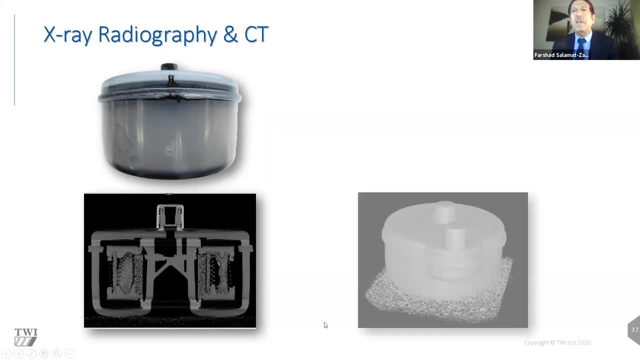 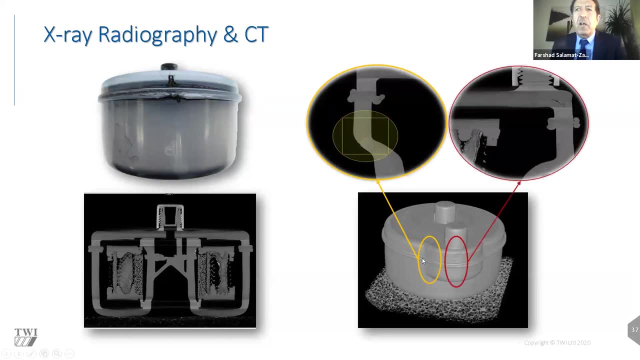 For example, we can see cracks here and we can see various features. Now, if I, if I try to enlarge on those and try to explain so, if I look at different corners of this- in here, for example, we can see a buckling has happened. 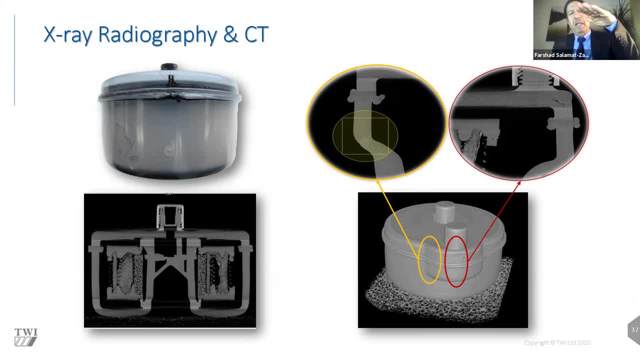 due to the high pressure, high loading pressure during the welding And we can see buckling happen. So we can get- we're getting- a stress whitening and the material starts to neck a bit at this point And we can see the misalignment of the lid to the base. 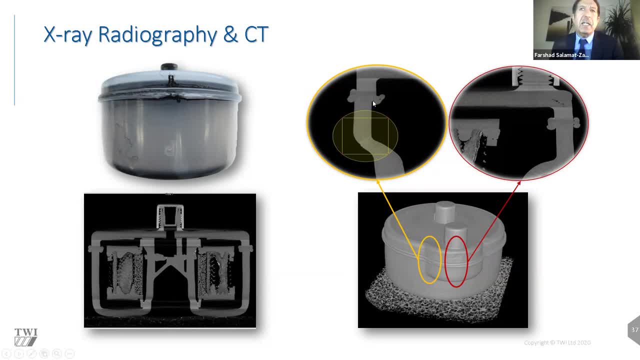 And we can see the misalignment And we can see the crack at the foot is propagating. You can see a crack propagation there. Now, if you look at this side again, we can see a void within the material, And so these are some information. 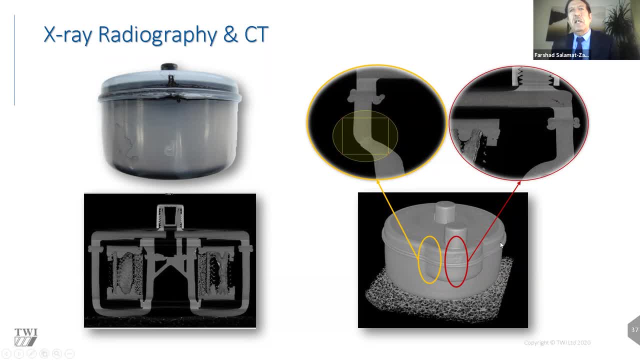 that you will not normally get with microtoning, because you're shooting in the dark, You don't know where to cut, You don't know that you can cut anywhere. You would be lucky to get to a point that you actually see it. 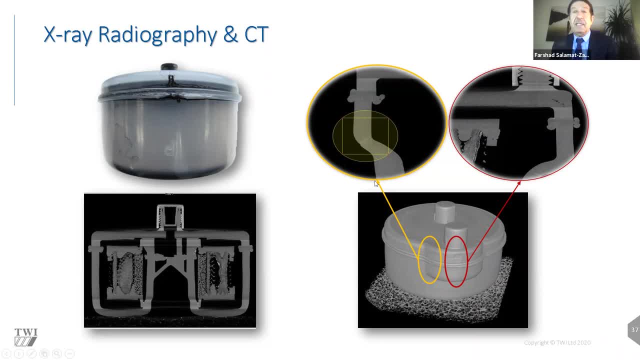 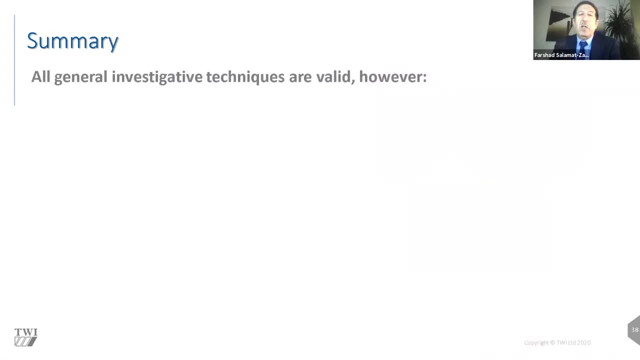 but you might actually miss this, But the XCT provides that information. So, in terms of the summary, to summarize, I wouldn't discredit all the standard techniques such as visual inspection, pressure test, leak test or that kind of technique, But I would stress that, for example, 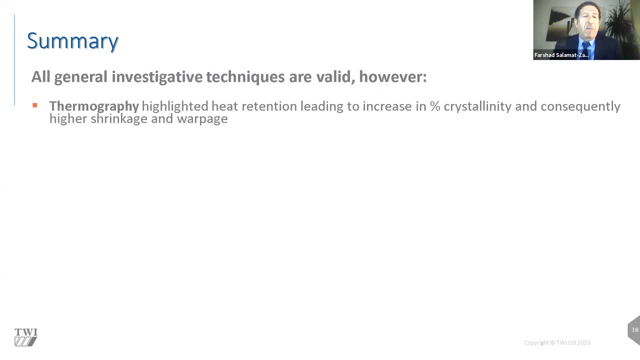 addition of thermography, can add a lot of values. We can understand the heat retention. We can understand how that heat retention can affect the, the crystallinity of the material which is going to lead to the shrinkage. Computer aided engineering, the modeling, 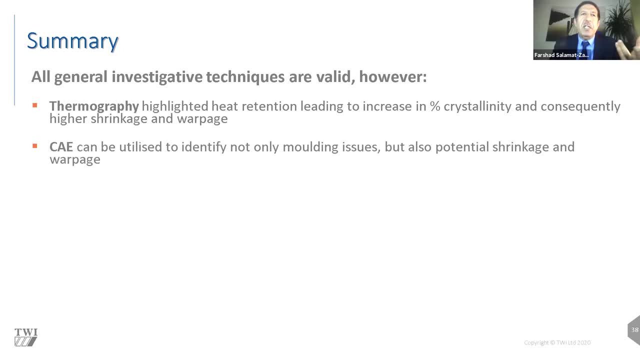 they see that it kind of predicted. it predicted a shrinkage and also predicted that the distortion were. when we tried to fit that, delete the base of the material, we could see that they could not fit it very well and it might've been done under a lot of pressure. 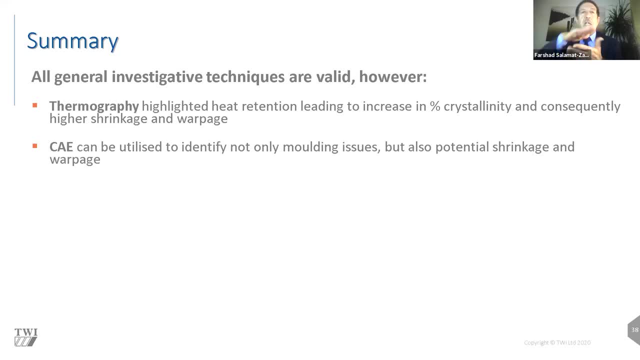 which, in time, it will put a lot of wear and tear on the tool. It will put a lot of wear on the tool. If you're, if everyone's changing the materials, you can see a我說 Yani fab αatRing matterțα and in갑writing meteringом. 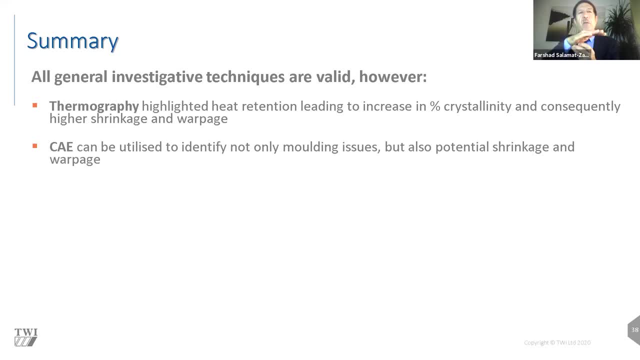 If they are not balanced properly, then you will put a lot of wear and tear on different locations of the tool due to excessive loading. But the CIE actually highlighted that The design rules are done for a reason. Obviously, there are guidelines for the manufacture of injection molding, for the tooling and for welding. 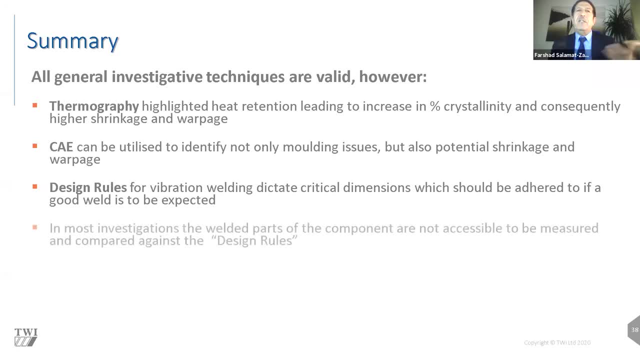 So they are set for a reason and we can use the design rule as a guide against the final product and see whether it actually matches the design rule and whether the component is fit for service. One major advantage of X-ray computed tomography is that the joint dimensions, which are normally hidden, can be analyzed. 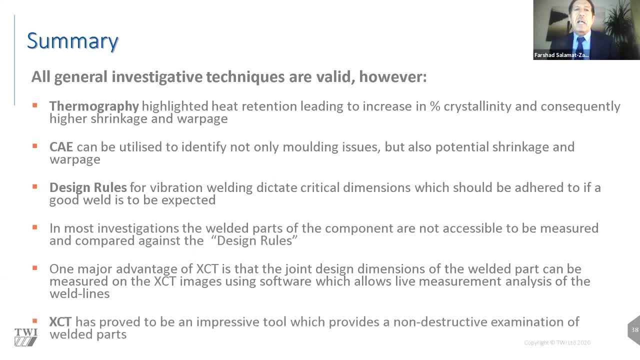 I showed that in one of my slides So they can be measured. And also the X-ray radiography proved, in my opinion, proved a fantastic tool, a very impressive tool that not only told us about the quality of weld, it also told us about voids, the void content. 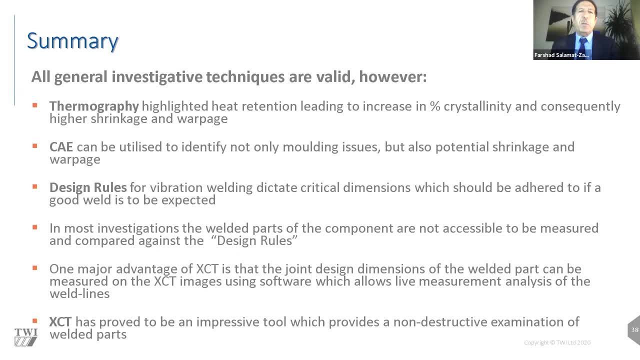 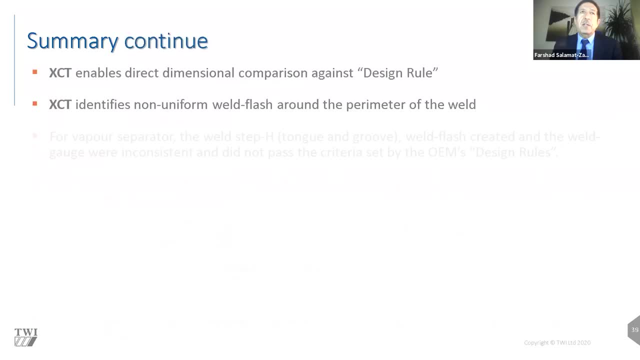 It also highlighted a lot of crack initiation, crack propagation. So there are certain things that you wouldn't see using other tools. So, Again, to continue, XCT enables direct dimensional comparison. I mentioned that earlier And also it highlighted the non-uniform weld flash across the perimeter. 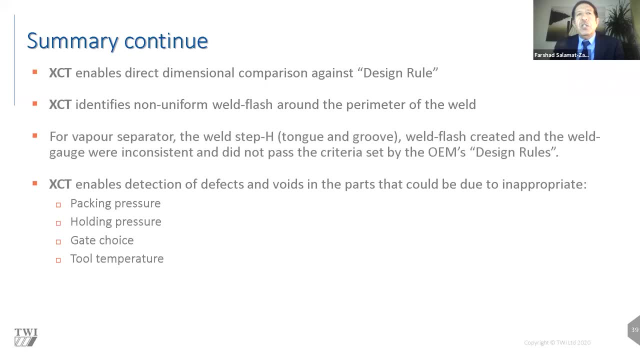 And also it highlighted other issues. I mentioned the voids, for example, That could, if somebody looks at that, they can say, okay, it might be injection molding issues. So let's look at the backing pressure, Let's look at the holding pressure. 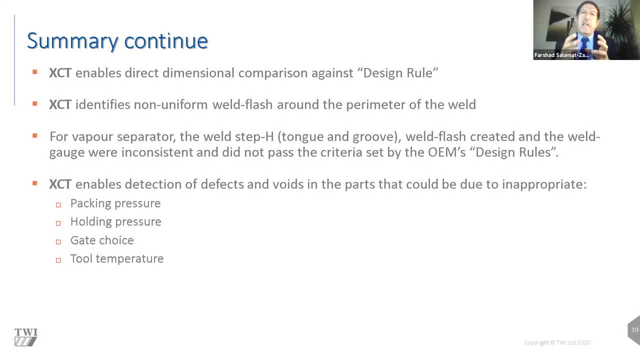 The gate choices, The tool temperature, All of those. they, as part of that issue cover diagram that I mentioned, or the failure mode analysis, you can try to identify what is responsible for this kind of failure that you are seeing. And obviously, information like this, the OEMs and other companies that consume good manufacturers and so forth- everybody they need to not only understand. 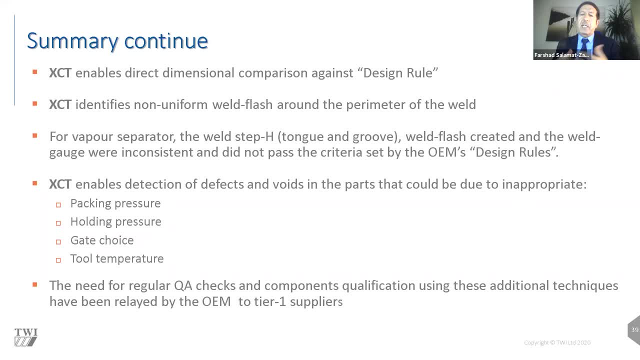 the issue. but they need to pass that information to their, to the supplier, so that the regular checks. it might not be on a daily basis, but it might be on a on a batch basis or it might be on a quarterly code, you know quarterly basis. so they need to run some sort of more detailed checks. 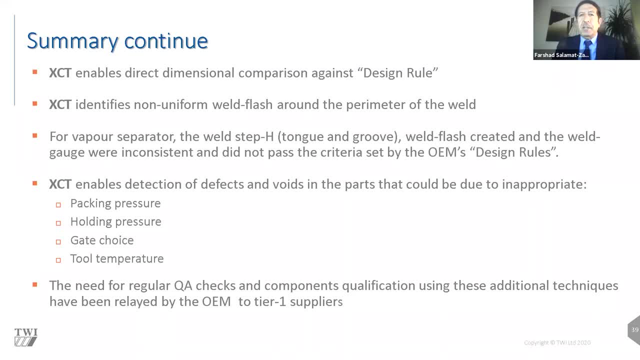 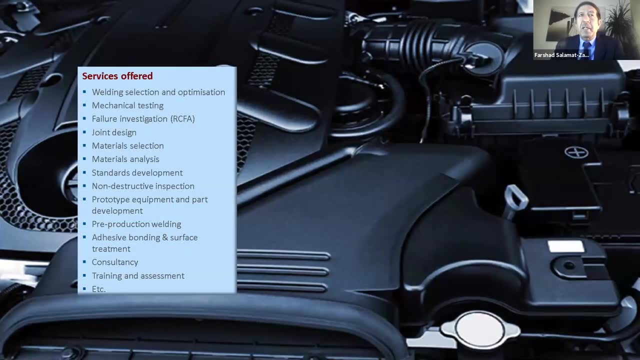 and just a visual, visual inspection or just pressure test now, in terms of the pwi and what we, what services we provide, from the weld selection, of welding process selection to optimization, from mechanical testing, failure investigation, material selection, joint design. the list is obviously is in front of you. you can see that we we try to support our member companies as much as we can. 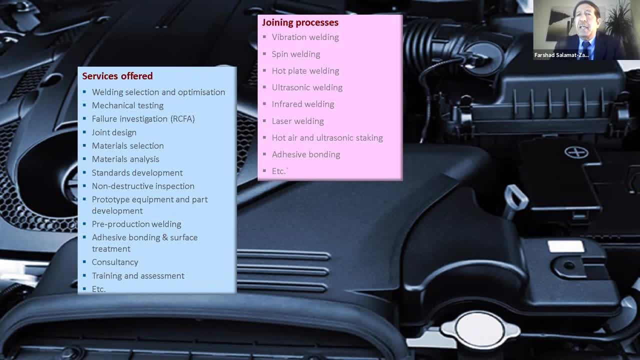 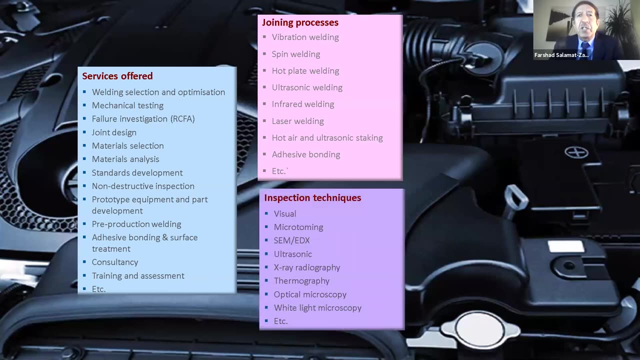 and we do provide. obviously, in terms of the welding technologies, we cover all the major. we have instrument and equipment in in-house to carry out trials and and so forth and process review for a lot of companies. in terms of the inspection techniques that we use, you can see that obviously we are, you know we are, we use visual, visual inspection, macrotoming. 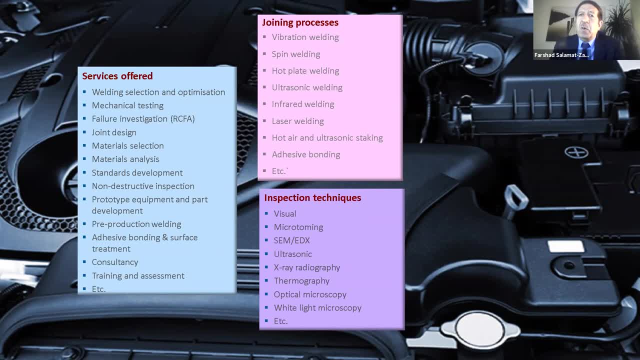 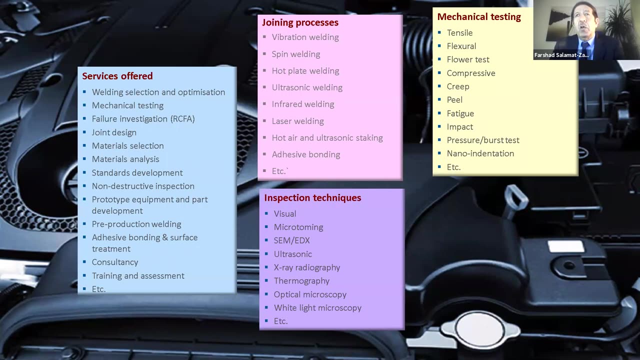 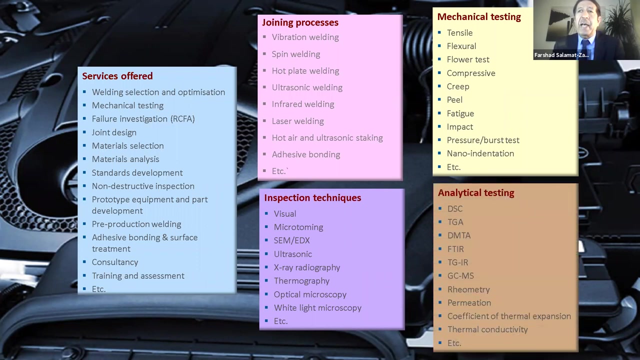 scanning, electron microscopy, ultrasonic and and so forth. so there's a lot of techniques, analytical techniques. obviously it's horses for courses, depending on what. what i'm investigating, different, different techniques will be utilized on level foreground. all those instruments and analytical capabilities we hold in-house which are, as i say, which are standardize or usc to do mechanical testing and if not, in terms of mechanical testing, whole range of from the coupon testing to the whole component testing. we can design rigs and fixtures, actually test the whole component, not just a standard coupon testing according to the standards. so those 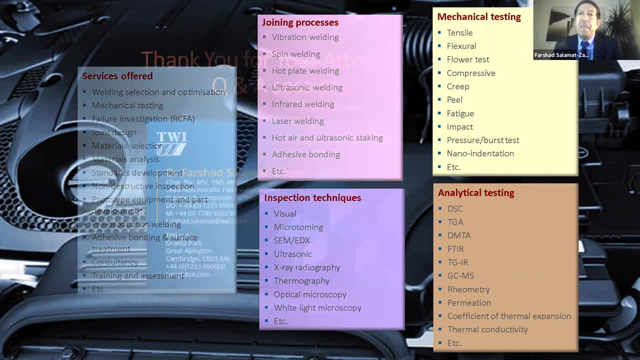 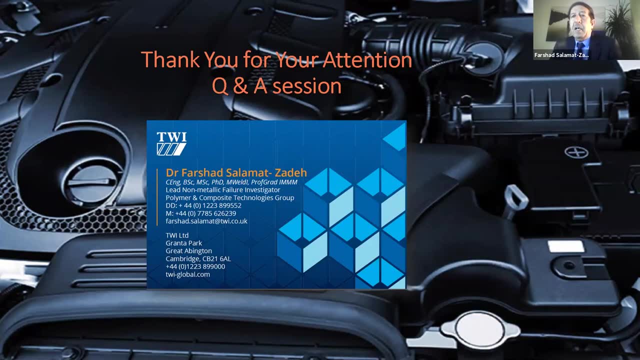 as I said, which are the extension of the resources of our member companies. so with that I end the webinar. I thank you for your attention and I'm open to any questions. thank you very much, Farshad. that was very, very, very, very, very interesting presentation we've got. 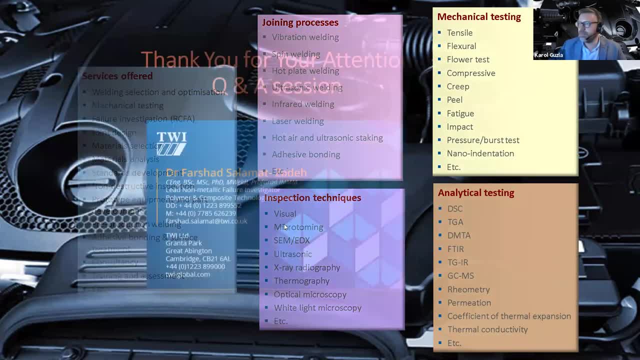 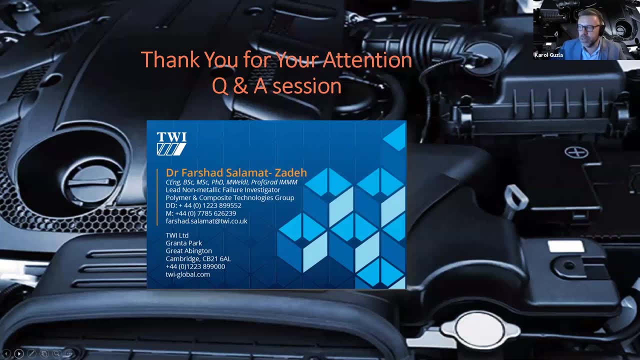 a couple questions. I'm not sure if we will be able to answer all of the questions. so first question is x-ray radiography of plastics? the same as the metals? basically, yes, the technique and the technology of procedure is the same. the main difference is that the metals- again, depending on which metals, metals are much denser, so the dense. 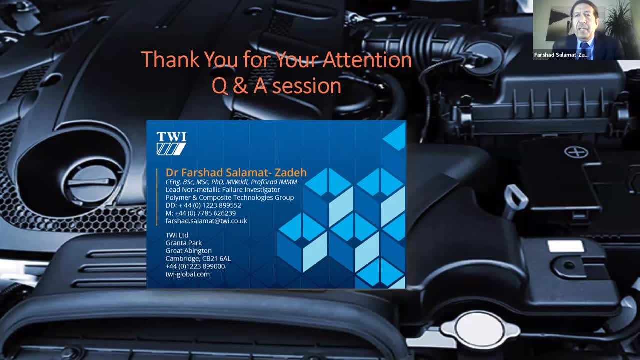 density is a critical part. So the operator, the x-ray operator, will sort out that sort of it. So yes, the thermoplastic materials or the thermosetting materials can be inspected with the x-ray radiography, as well as the metallic ones, for sure. 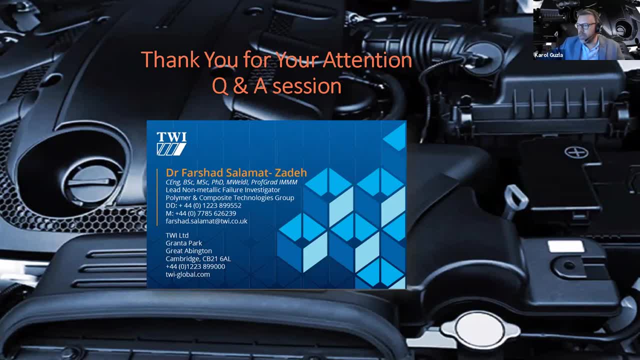 Okay, thank you. We got another question about the x-ray. Can you inspect plastic parts with metal inserts by x-ray? It can. Again, the danger here is the issue with the metal to plastic density, Obviously as a component. some of the components are. 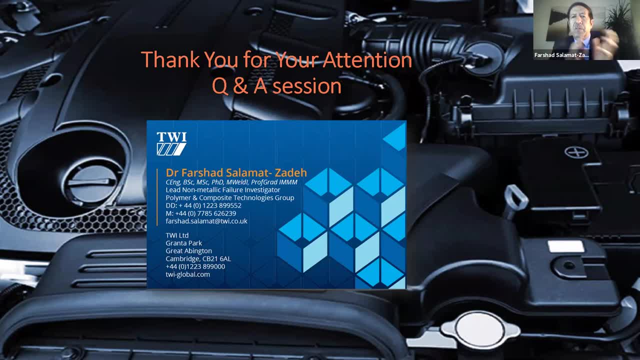 done So when we inspect them, the plastic components we can inspect easily. When we get close to the metal insert and buses and so forth, you might get a lot of backscattering and a lot of, you know, a lot of. 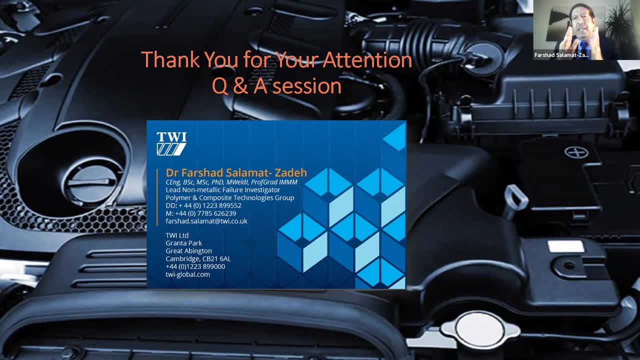 a lot of flashes of light around the vicinity of that, So the interface, which is quite critical, between the metal and the plastics might be a bit obscured with various flashes of light there. But however, saying that, although it's very difficult, as I said, due to the 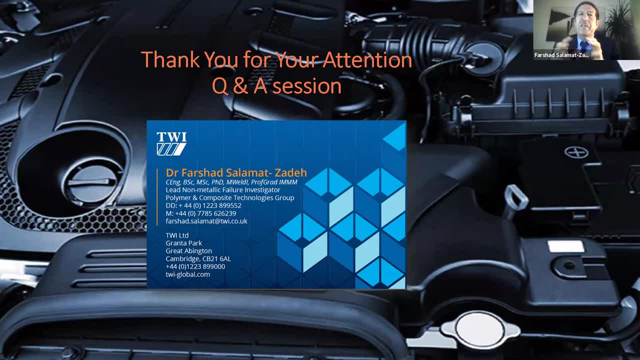 change of density. but there are ways that with the software they can make certain adjustment that they can, you know, ease that slightly so that you get a better view of that. Okay, Thank you. Another question about plastic welding: does TLB provide training courses? 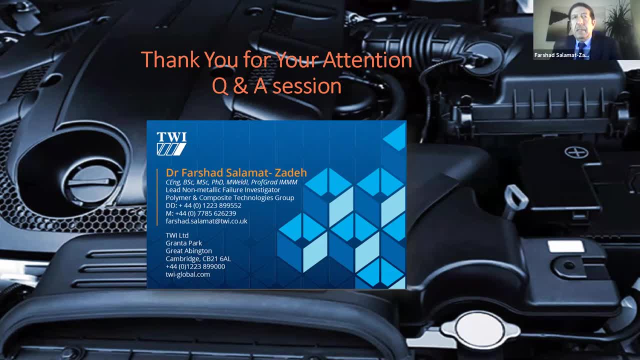 on plastic welding. Yes, we have a training course which is a three day training course and we run it three times a year. This year because of the COVID, we did not run it Again because of social distancing and all that, but we aim to run it as of next year. The course covers most. 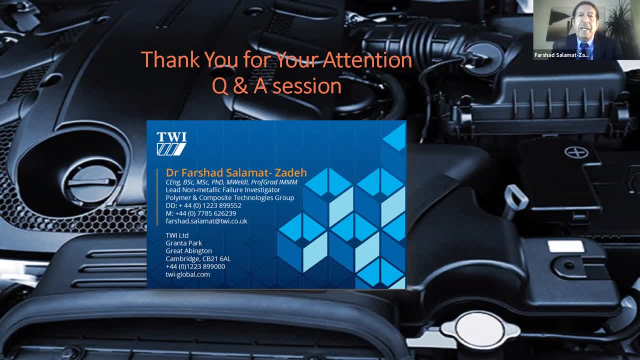 most of the techniques that are relevant to thermoplastics. We touch on some of the manual processes which are not for the, which are not really for the, let's say for the automotive or consumer good materials such as hot gas welding, which are more, or extrusion welding, which are 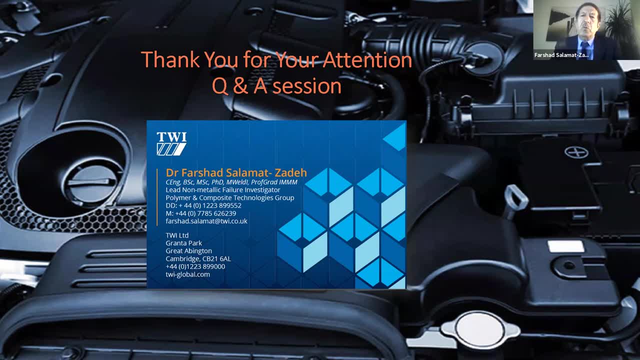 more of a manual process. We have one or two modules that covers those as a combined module. but things like ultrasonic welding, laser welding, hot plate welding- all of those are standalone modules and they're covered in a three-day course which is a mixture of theoretical 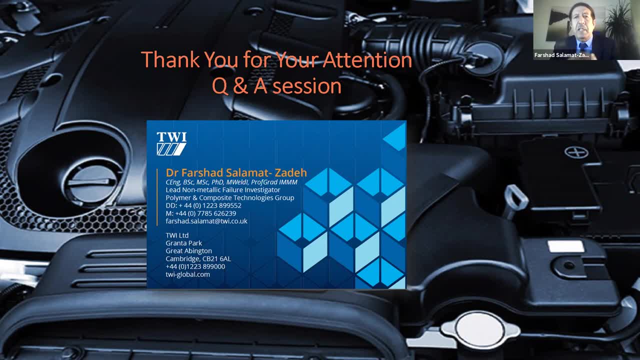 and also practical practices. So if anybody is interested, if you get in touch with me, I'll try to provide you the right information. Perfect, Do we have the time for a couple more questions? Farshad, Yes, yes, please. 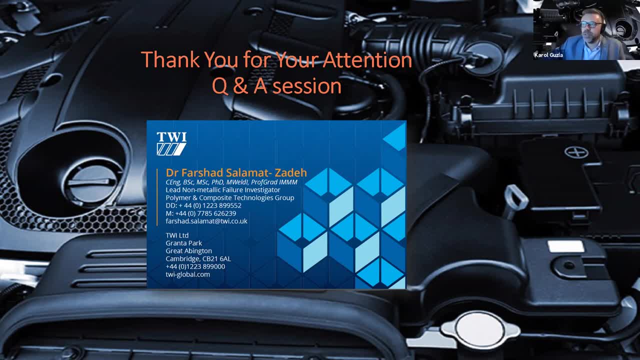 Okay, There's a question about ISO standards. Are there specific ISO standards for joining polymeric materials? Well, there are lots of international standards- ISO and ASMIS- on welding of plastics, but a lot of them refer to geomembranes and plastic pipe welding. 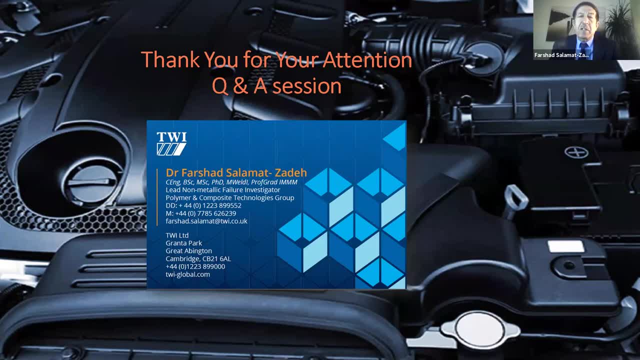 rather than the plastic component. As a result of our activity and our involvement with this investigation, and also collaboration with a few OEMs, automotive companies and consumer goods, about four years ago we started looking at setting up a BSIS standard- British standard- 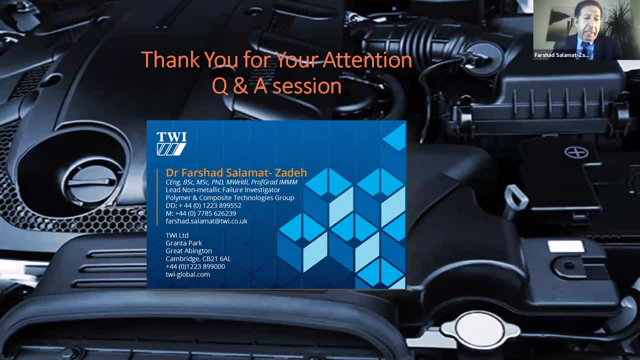 on welding of plastic components And I forgot the name of the standard, but I can forward it by email to when we share the presentation. I can forward the link to the BSIS standard as well. Basically, there is a standard, the British standard. 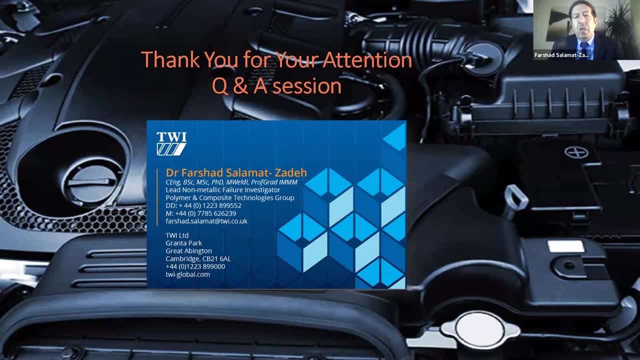 that was developed, which was released over a year and a half ago. So that gives guidelines to all major welding technologies. The aim is that obviously the next step is for us to take it to the European and then from the European, then the next stage will be to take it to ISO standard. 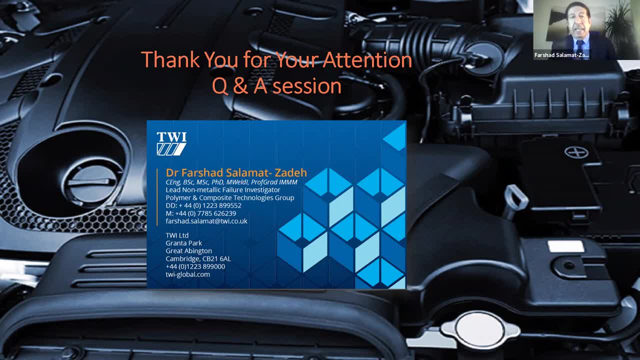 Okay, But it is a as it stands. there is a British standard that you can, you can use and refer to, for sure, But, as I said, we will pass that information with the presentation to you later. Fantastic, Thank you very much. One more question about inspection techniques. 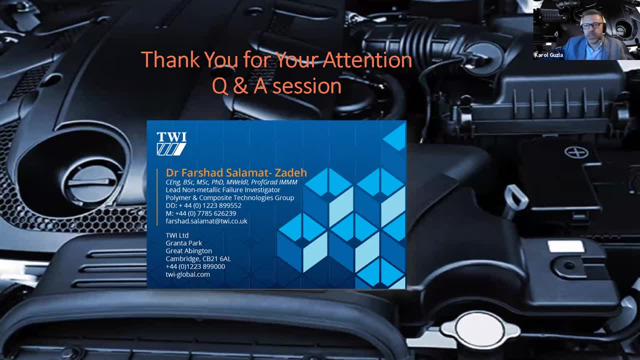 What is the main advantage of thermography technique? Well, as yeah, I mean the thermography is. again, it's not commonly used by by by many, But I think this is something that that is quite useful, And I hope that I demonstrated that in the presentation. 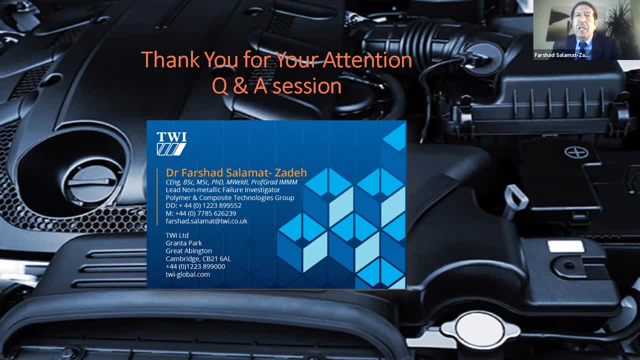 Basically, it provides hidden information about the heat retention within a material, within a product, after it's been welded or after it's been injection molded, And even during the welding process, post welding. you can you can carry out the thermography, where you can see different heat. 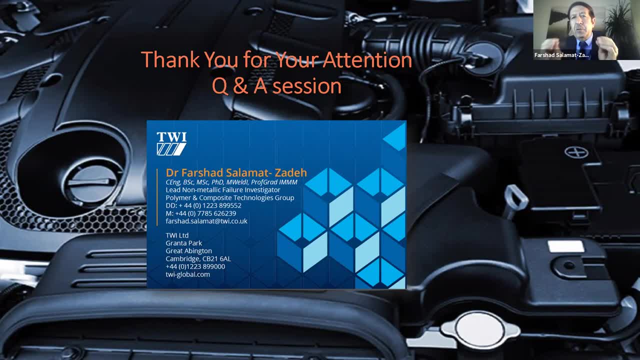 Heat retention And if you don't get uniform heat, heat dissipation and cooling down, you end up with a variation degree of crystallinity which leads to the different shrinkages around the product And that also leads to different workages, which is going to cause quite a bit of headache in terms of your many 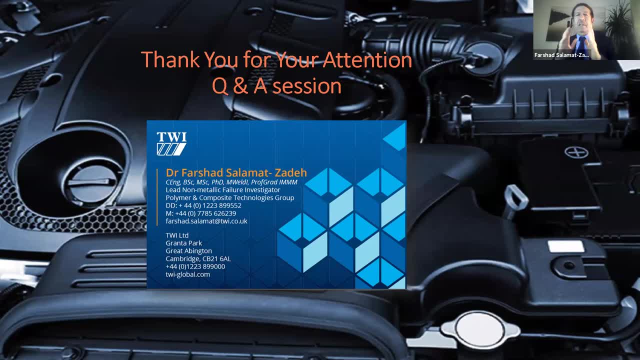 many try to weld them together because they don't mate The male and female part of. they don't mate properly, They don't fit properly, Or even if they do and you have to do under a lot of loading, then the chance of material failing is exaggerated, obviously because of that. 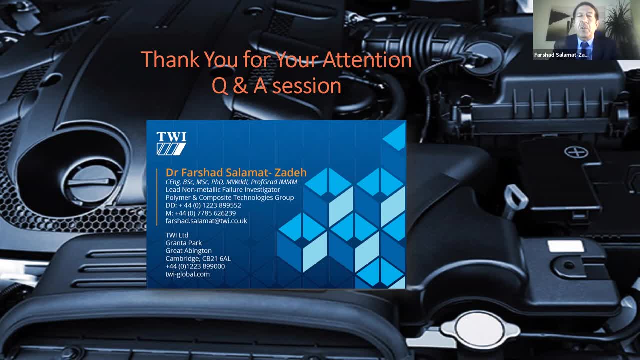 So it's quite a unique but very important tool to use for sure. Yeah, Thank you very much. Thank you very much, Farshad. Yeah, it's thank you for for for your amazing presentation and for the question you've managed to answer. 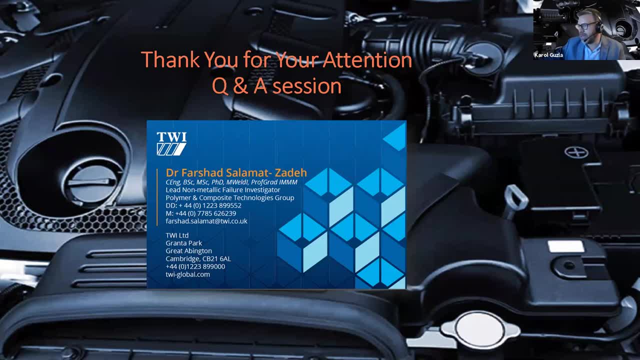 I think we're running out of time now here, So we will bring the webinar to a close. Let me just add one thing: that obviously, the questions that have been put forward we haven't had a chance to respond to them, We will respond to those And again, we will either individually or as a group. 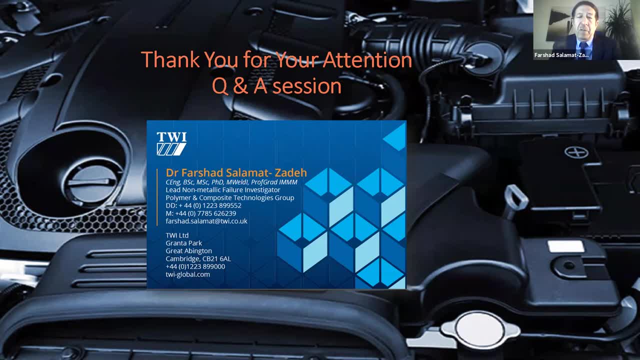 we can accompany those answers by email when we send the presentation out as well. Thank you for your attention. Yeah, Yeah, Thanks. Thanks again for for for everyone for attending today. We will try to distribute the recording and PDA version and we'll get back back to you with unanswered questions. 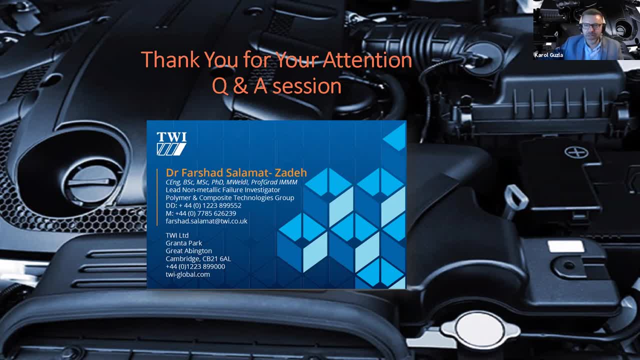 And also as it is one of the last webinars this year, we would like to wish you Merry Christmas and Happy New Year. All the best to all of you. Thank you, Merry Christmas, Happy New Year to all. Be safe, Bye, bye. Thank you. 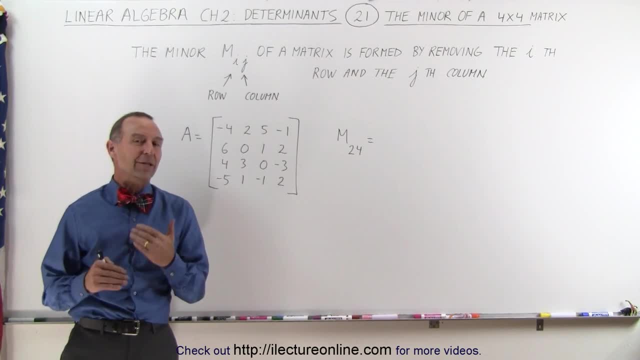 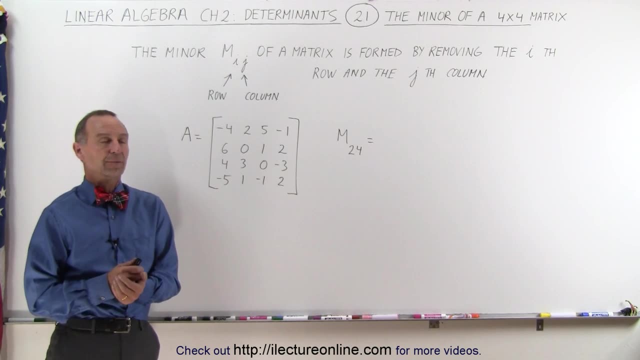 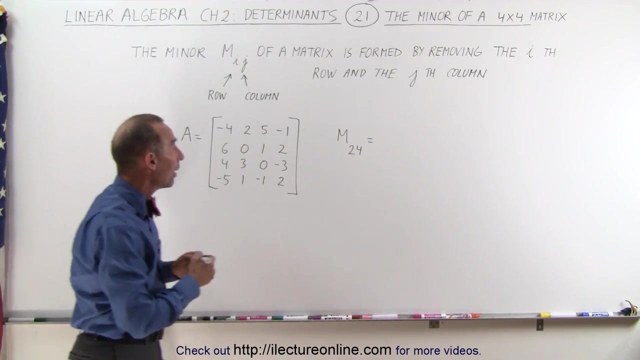 Welcome to ElectronLine. Just to make sure we don't have any confusion with finding minors here we're going to take the minor or find the minor of a four by four matrix. We're trying to find M24 of the matrix A. Again, what we do is we repeat or copy the matrix. 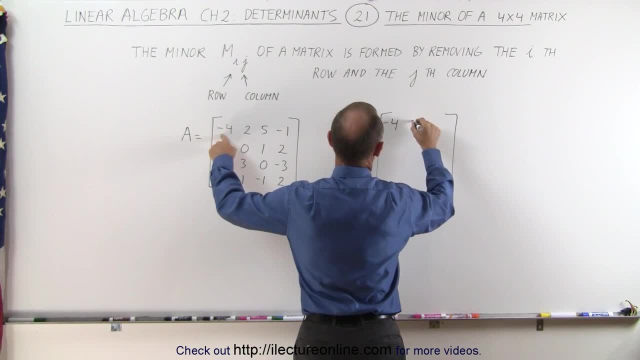 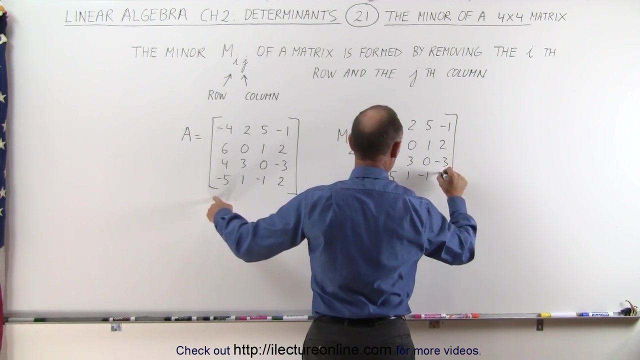 We put all the same elements as before. We have six- zero, one, two, four, three, zero and minus three and the last row, minus five, one negative one and two. And then here we realize that this is the row we want to. 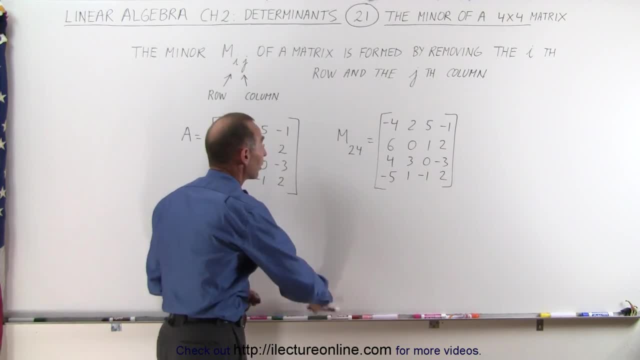 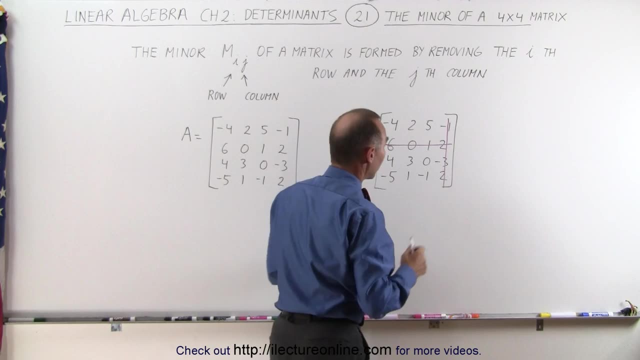 get rid of, and this is the column we want to get rid of. So we take another colored pen. the second row- completely, is gone, and the fourth column is this column right here. Now, this is the first column and it's basically done.